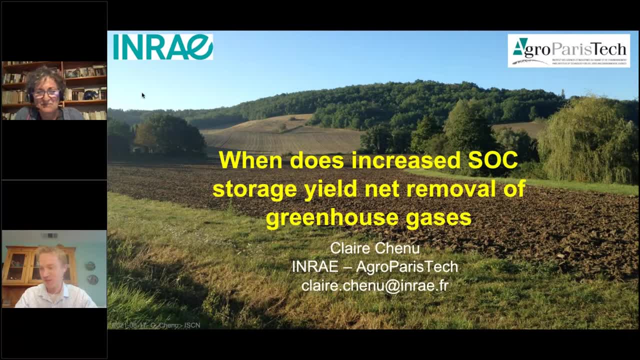 and many thanks for that, Claire, for joining late in your day. as it is, Claire is the Research Director at INRAE, which is France's National Institute for Agronomic Research. She's also a Professor of Soil Science at AgroParisTech and the Vice Chair of the Scientific and Technical Committee of the Four Per Mill Initiative. 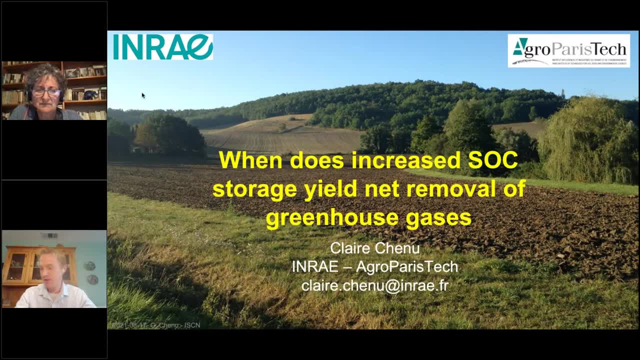 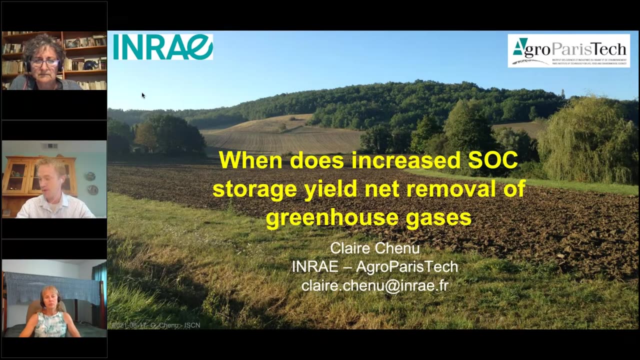 The second speaker we'll have today, midway through the webinar, is Jane Johnson. She's a scientist and research leader at the USDA ARS in Morris, Minnesota. She's a Fellow of the American Society of Agronomy and she's a US Co-Chair of the Global Research Alliance, an international body. 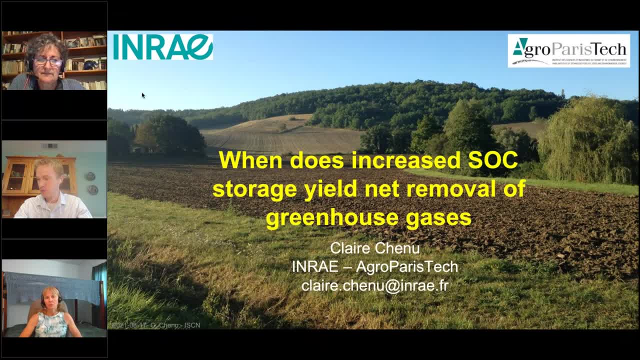 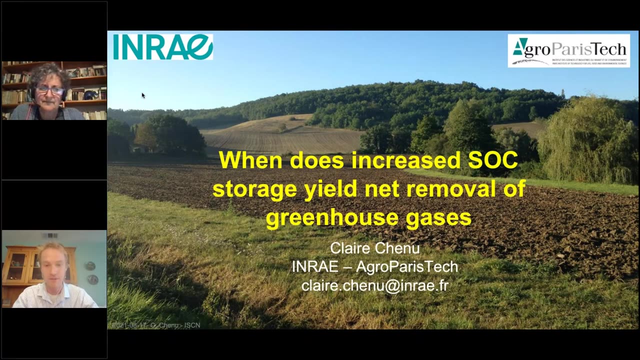 that is, promoting research to reduce ag emissions. And with that I think we'll lead into the first talk. Claire Chenu will begin addressing the question: when does increased soil carbon storage yield net removal of greenhouse gases? And take it away, Claire. 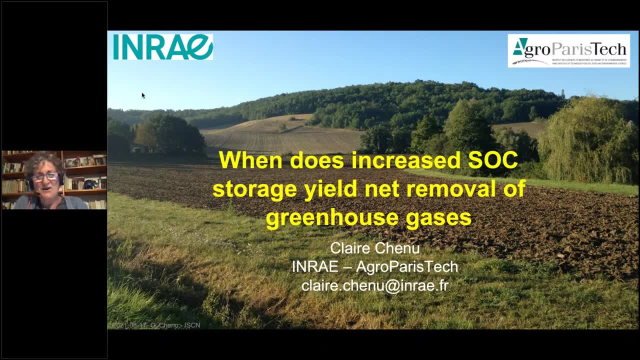 Thank you, So good afternoon everyone. So we were just discussing that this landscape could look like Northern California. Well, it's actually a landscape from Southwest France, and I'm talking to you from Paris area. I live in Versailles, So I'm very pleased to be with you today. 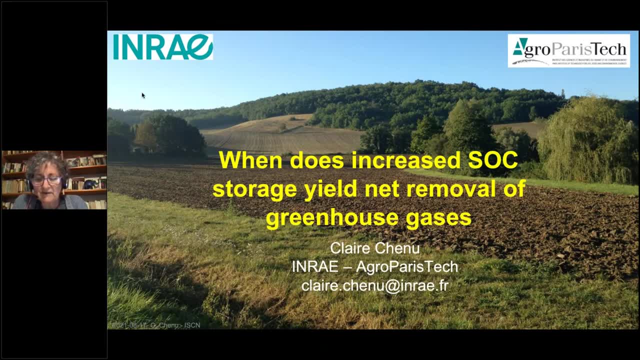 because I am part of the Otatou microclimate policy committee And actually I am someone working so in France at NRA on carbon dynamics, or sobre did I amando enIGH fluidmytème d'arbore y starto en Ilurfé enbartée en� husqvasi d'agricultores agriques. 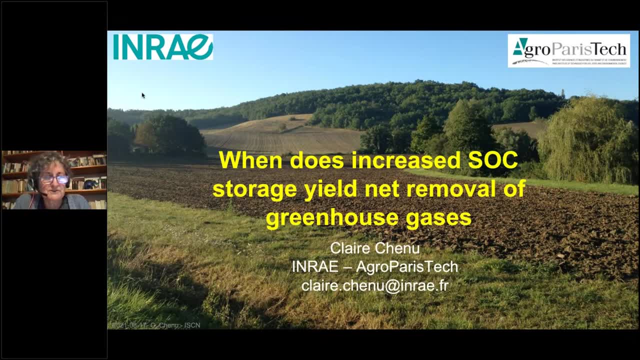 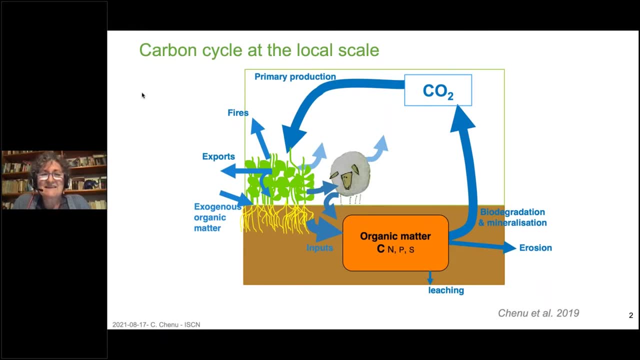 en hydroponía y césar et en salle de stockage de carbone agroecológica in agricultural soils. So this is basically what I'm working on and well, you know that in the different carried out a prospect of an agro-agriculture. 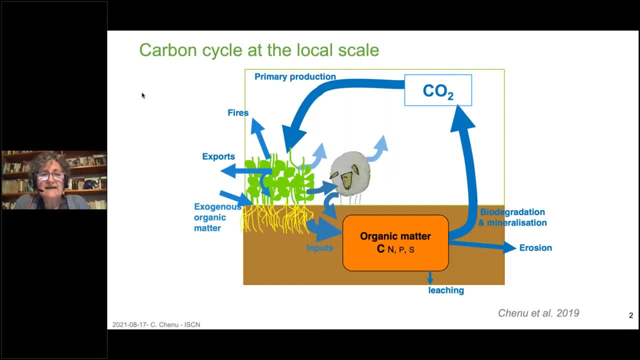 component. So these are유 con feel at this centre. you know that in the different various components of the carbon cycle at the local 2016, 10 years ago, increased and reduced the local scale can affect soil organic carbon storage. that dinc é sため loses aura. cet é RangerENS de compositions. 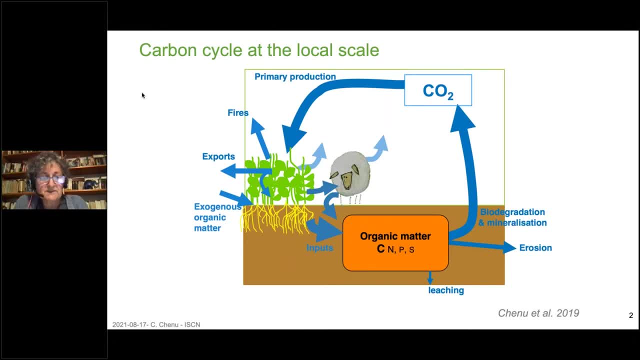 storage, that is, the increase or the decrease. the increase of stocks and the increase carbon stocks come from a positive balance between inputs and outputs and that the current state of knowledge shows that it is. what is most efficient is to increase organic carbon inputs to soils compared to trying to reduce uh outputs, and these primarily through enhanced biomass production by the agro. 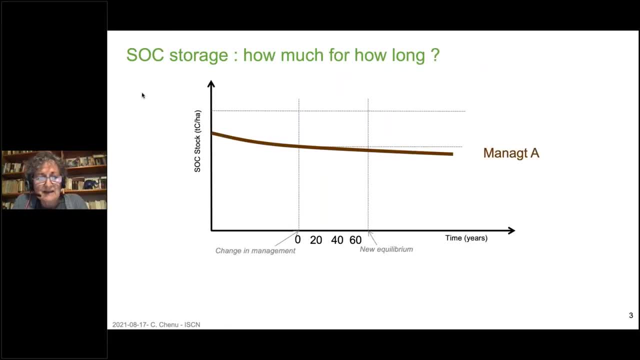 ecosystem and if we consider this at with time. so let's have a very simple graph where you have these organic carbon stocks. as a function of time, let's set a baseline. this would be actually the baseline of average evolution of organic carbon stocks in mainland. trends are very slow, low slope decrease and it's more or less the same across Europe. 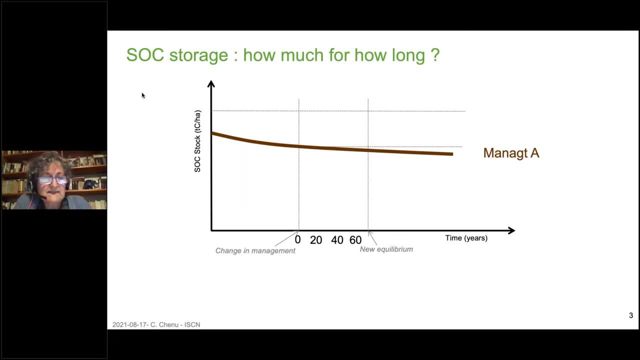 in average. So this is the baseline. Now, if we implement a carbon storing management option, for example implementing cover crops in the rotation, the carbon stocks will increase and will somehow plateau, reach to a new equilibrium. Storage is limited in soils. 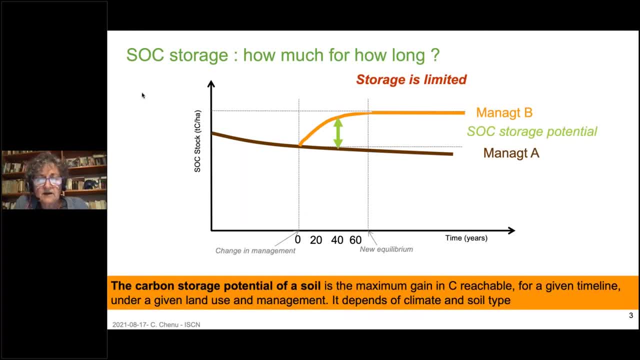 If another, And this defines the carbon storage potential. So the carbon storage potential is the maximum gain in carbon reachable for a given timeline. For example, my green arrow is located at 40 years under a given land use and management option. It depends on climate and on soil type. 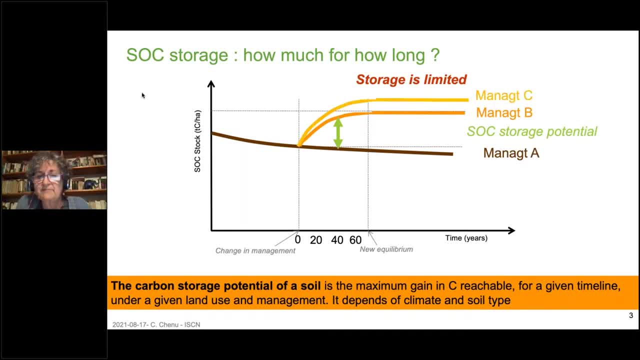 There's no general carbon storage potential. It is context dependent, And if another management option is applied- let's consider, for example, agroforestry- maybe the new equilibrium will be higher. What you can also see on this graph is that storage is low. 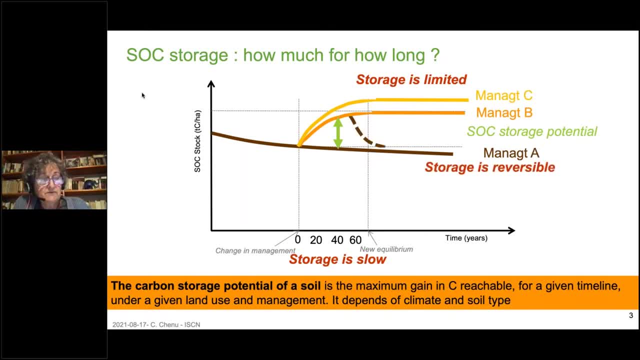 It takes years, decades, That it is reversible if the management option is reversed to the initial one, And that what is most detrimental is changes in land use, For example returning permanent grassland. the loss of carbon is then rapid and huge. 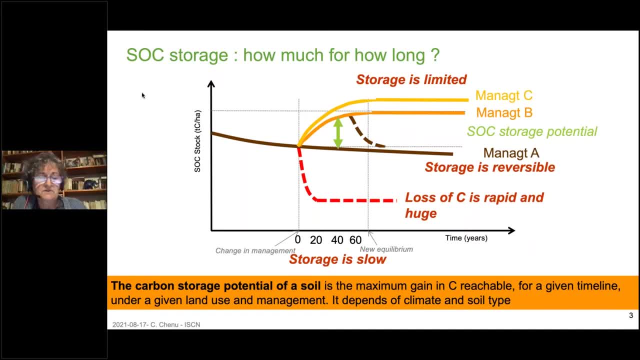 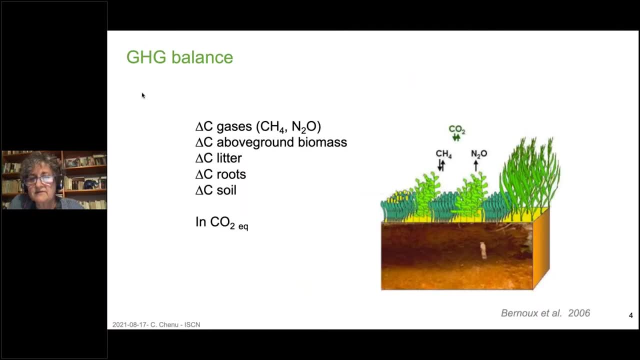 So this is for carbon. Well, the general feedback. So the question here is net removal of greenhouse gases. So a balance needs to be made, A balance between the fluxes of non-CO2 gases, methane and N2O, and the balance between variations. 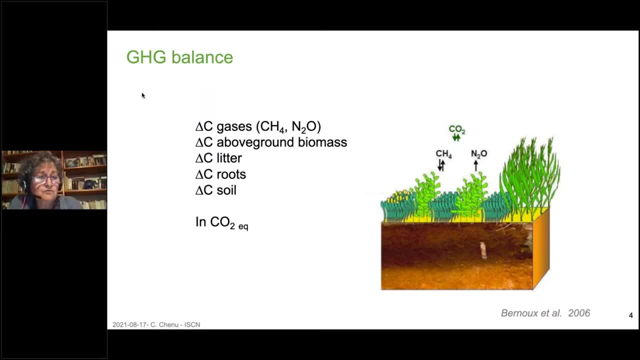 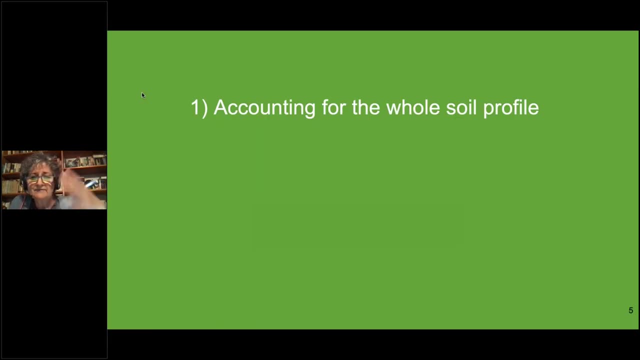 of above ground carbon stocks in above ground biomass, litter, roots and soil, all expressed in the same unit CO2 equivalents. Considering the global warming potential of the different gases, CO2 being the reference Now I would like to make, I have found that, if one wants to, the carbon storage increased. 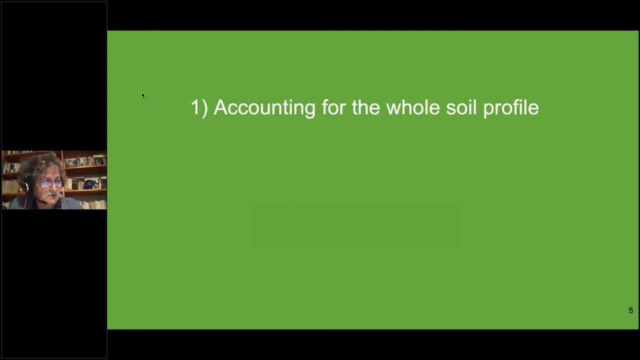 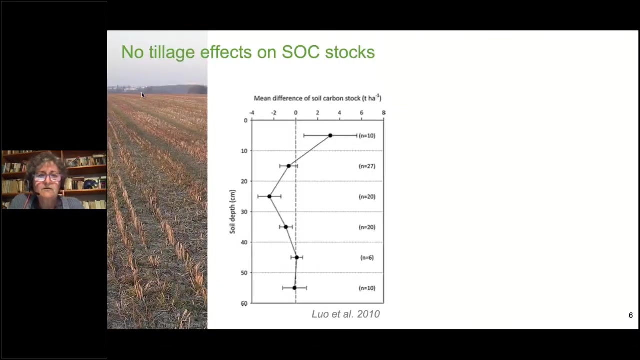 stock storage measurements, or well, increased stock storage, to yield the net removal of greenhouse gases. there's a need to account for different things, And I will give you examples for the four of them. First is accounting for the holes. So, for example, if you look at this graph, you can see that this graph is a graph of. 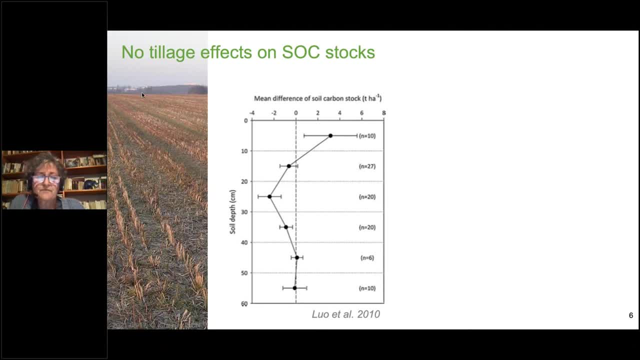 the total soil profile And quite classical example is the effect of no tillage on soil organic carbon stocks. This is a graph from a meta-analysis from Luo et al that showed very clearly- and but there has been a number of meta-analysis and studies- that with no tillage the concentration 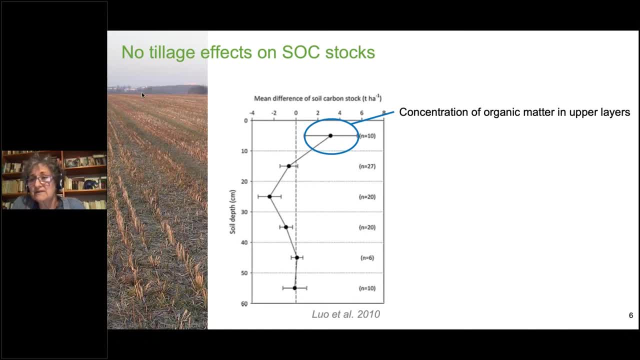 of organic matter and organic carbon stocks increase in soil upper layers, while they tend to decrease or not. They tend not to change below the upper layers, so that the balance- and it was the case in the meta-analysis of Luo can be- can be nil. 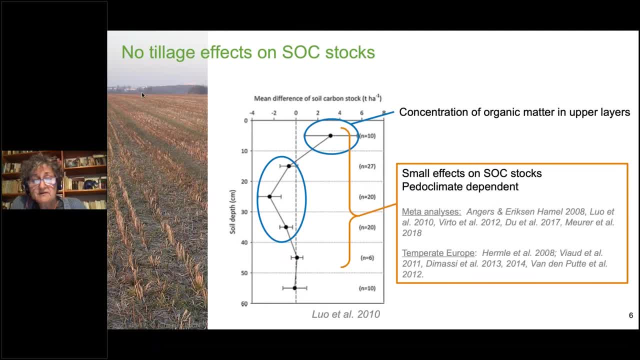 Overall, there are small effects on soil organic carbon stocks if you consider the whole soil profile and this is pedo-climatic, pedo-climate dependent. it is especially true this very small effect in temperate conditions. So to so, if 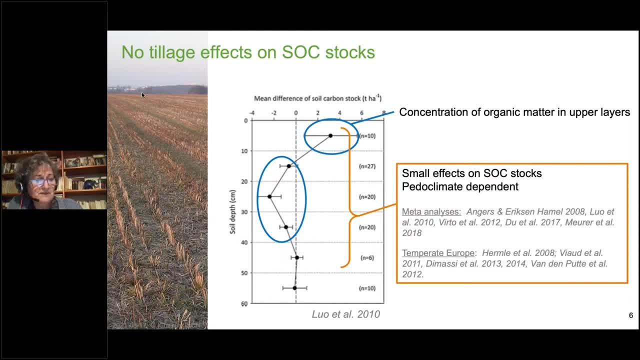 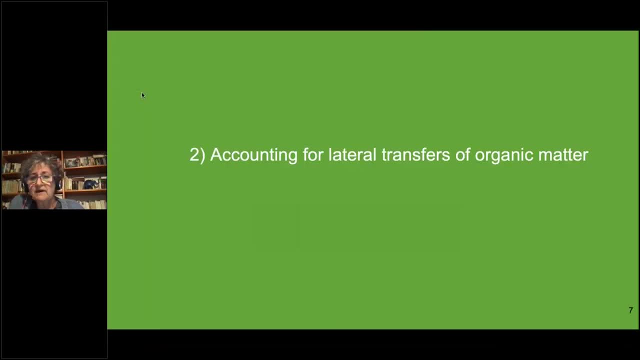 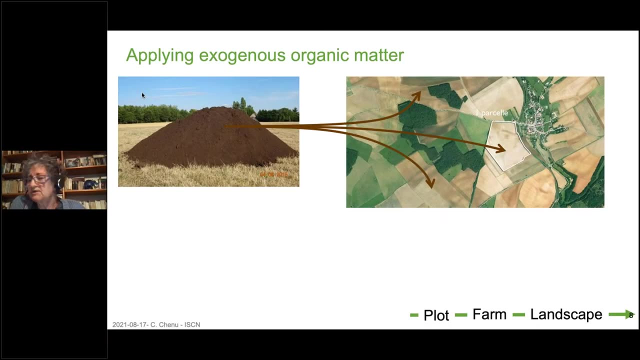 For the observed carbon storage to correspond to a net offset of greenhouse gas emissions, there is a need to consider the whole soil profile. There is also a need to account for lateral transfers of soil organic matter, And here I am essentially thinking of exogenous organic matter. 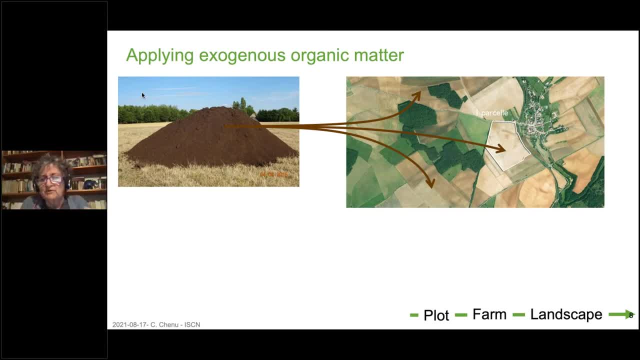 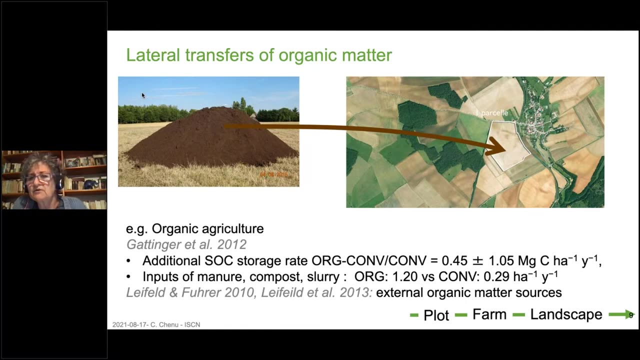 Let's consider one situation where a given resource of manure was applied is applied by a farmer distributed between three plots, As I shown on this photograph, and one day he decides to change and he applies the manure on the whole manure on only one plot. 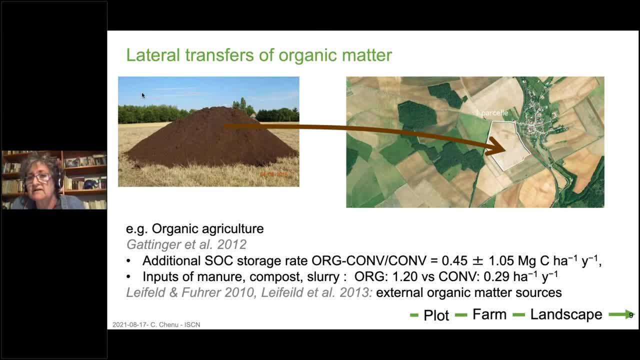 In this plot, the carbon content, the carbon stocks will increase. carbon storage will increase, but carbon, the net uptake of CO2 from the atmosphere at the landscape level, will not change. Carbon has just been transferred from one place to another, and these for example: 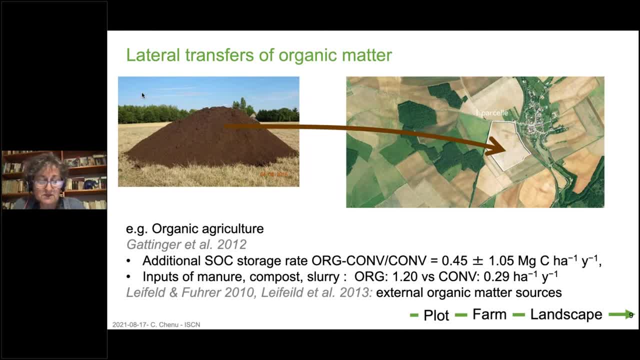 has raised. So we can, we can see here to that fiscal year claimed to be one of the most significant, non-faultier steps. So now We can, quickly, Let's look at that We can. we can get back to that program. 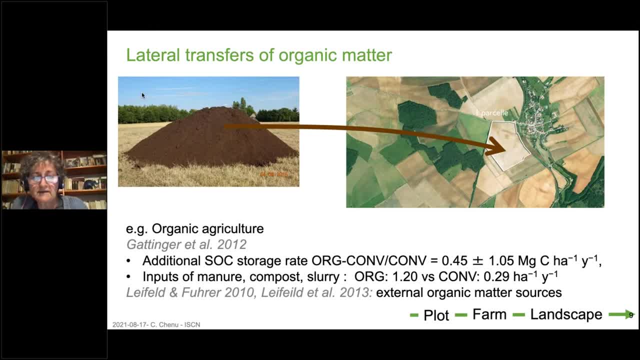 We can get back to that and slurry And, as was discussed and shown by Liefeld and others, in many cases the external resource, the organic matter resource, came from outside of the plot, outside of the farm. even So, it's just transferring organic matter through the landscape, not net carbon uptake, So not net. 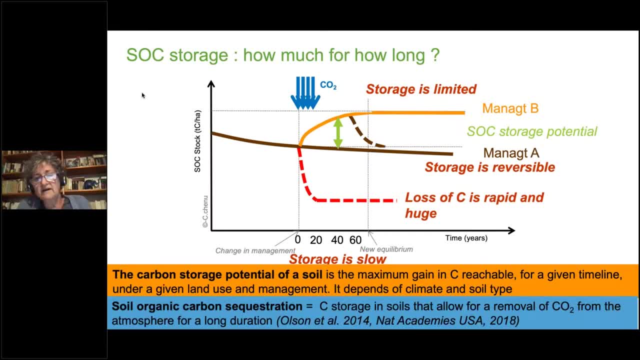 carbon sequestration. So soil organic carbon sequestration has a different meaning than soil organic carbon storage. It corresponds to the storage in soil that allows for a removal of CO2 from the atmosphere for a long duration. So in my example of moving around manure there was 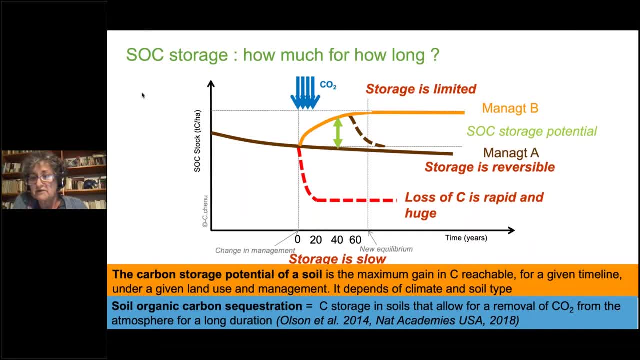 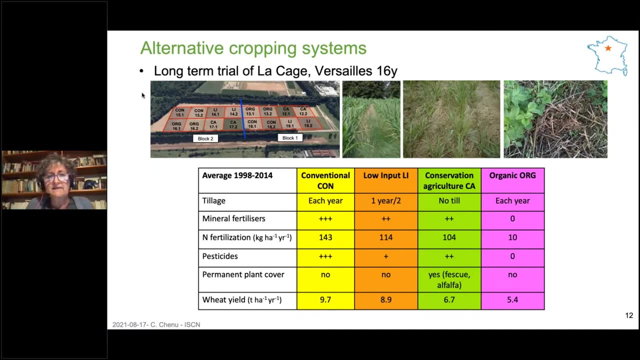 no additional carbon sequestration, but additional carbon storage in the plot that received all the manure, So accounting for lateral transfers of organic matter. There is also a need, of course, to account for N2O emissions, And here I will use an example of a long-term experiment on which 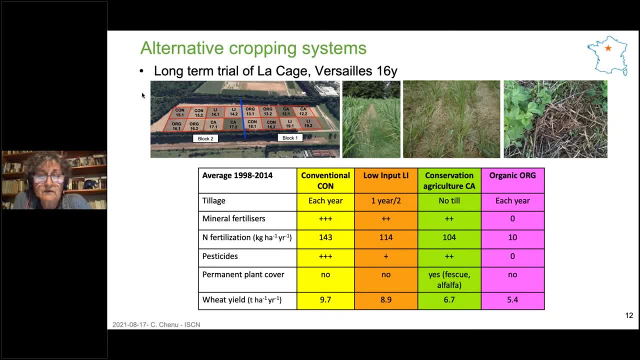 I work where in rotations with cereals or wheat one year over two, we compare since 1998 different cropping, alternative cropping systems that are compared to a conventional one And you see the main characteristics here. So we have a low input system with reduced mineral fertilization, reduced tillage. 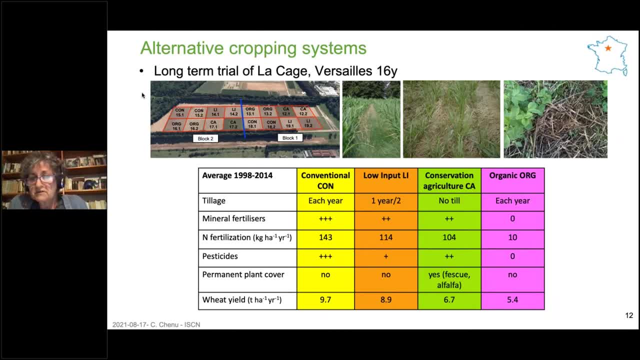 that leads to slightly reduced yields. We have a conservation agricultural system with no till, with also reduced mineral fertilizer, based on the low input system, with a permanent coverage of the soil by a plant, and it's now alfalfa And it also has yield. 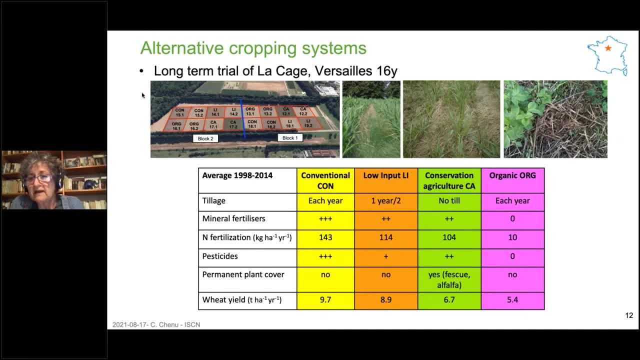 that are lower compared to the conventional and an organically managed system that receives no manure, no compost. It is actually representative of some systems we observe at farmers place in Paris area: The stillage each year. of course, no mineral fertilization. 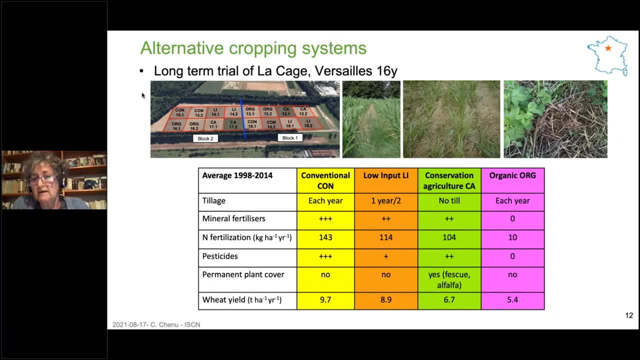 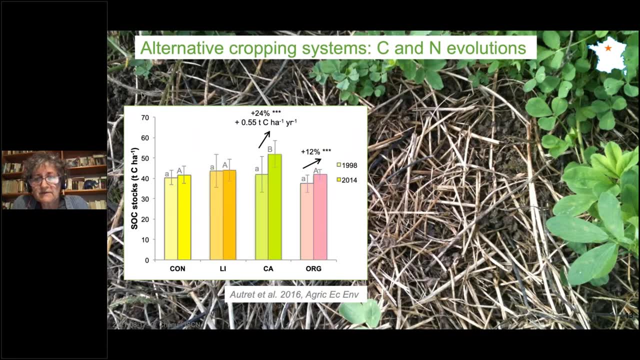 but there's a wide use of legumes in the rotation and lower yields. Now we compared the organic carbon stocks at the start of the experiment. We compared them again in 2014.. We just remeasured them but didn't plot the new results, And what we observed is that there was a slight 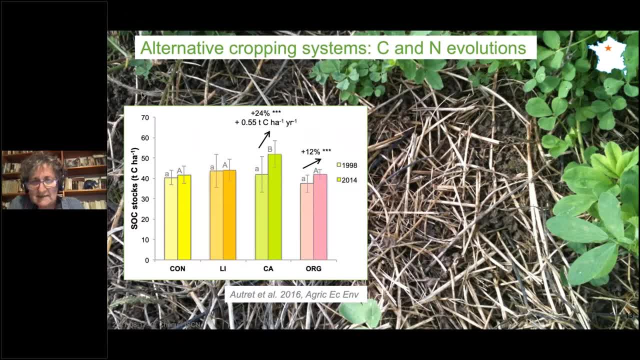 increase of organic carbon stocks in the organic system, but with very low increases. with low increases, but a good, an important increase in the conservation agricultural system And actually we were able in this trial to show show that the increase was could be completely explained by the additional. 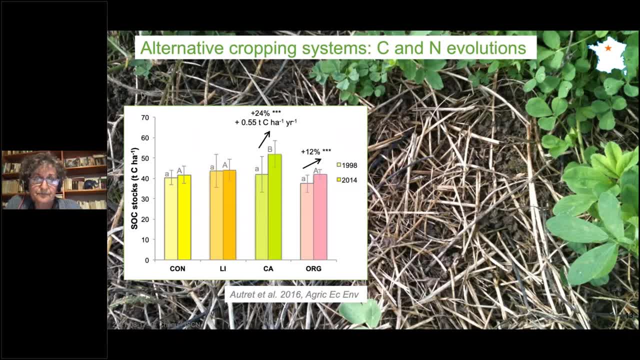 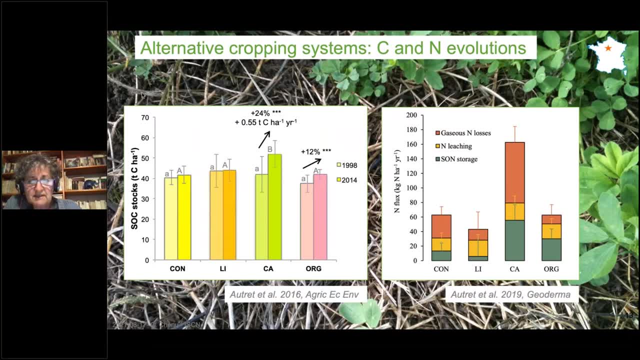 biomass due to the alfalfa. Bénédicte Autré also measured nitrogen leaching. well, she estimated nitrogen leaching- you see doesn't vary much between the different system- and she measured over two years continuously the N2O emissions and she found that they were much larger. 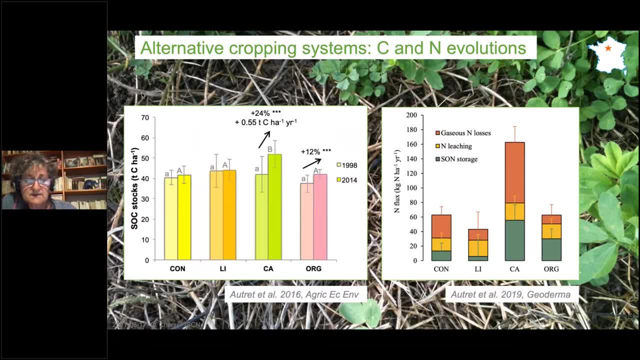 in the conservation agriculture system, compared to the conventional and to the low input, The amounts of mineral nitrogen added, of mineral fertilizers are the same as in the low input system. so it's not that, and the explanation is actually that there would be additional denitrification because of this mulch. 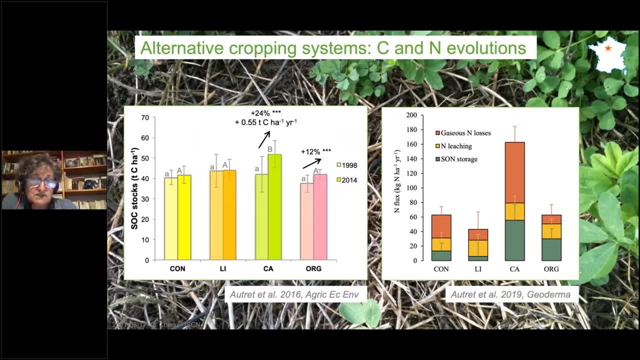 that remains humid without the low C2N alfalfa over the year, so this would create conditions and the soils are slightly acidic, so this would create conditions for additional N2O emissions in the conservation agricultural system. So this is one case study. Now, if we consider different management, 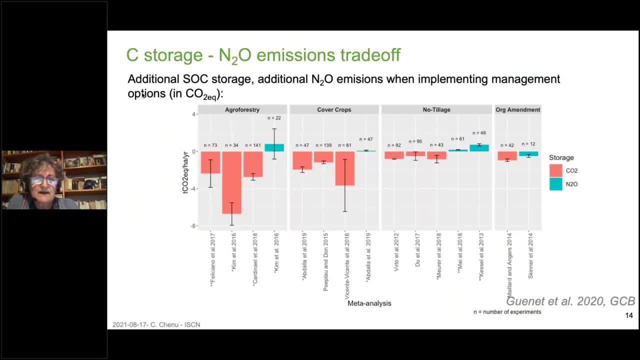 options. Guenet et al assembled different meta-analysis where had been quantified either the additional- so organic carbon storage or the additional N2O emissions when implementing different management options. it is actually very rare to find meta-analysis that compiled the two types of information, So 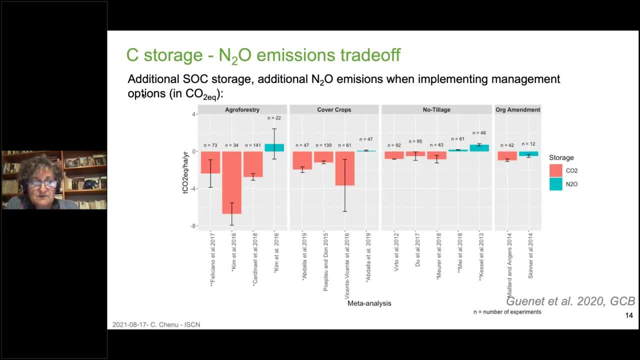 it's usually separate ones. The carbon storage is represented as negative an uptake of CO2 from the atmosphere, so it's in CO2 equivalent. the N2A emissions are represented also in CO2 equivalent, but is in green. You can see that N2A emissions can decrease the positive effect, the effect of 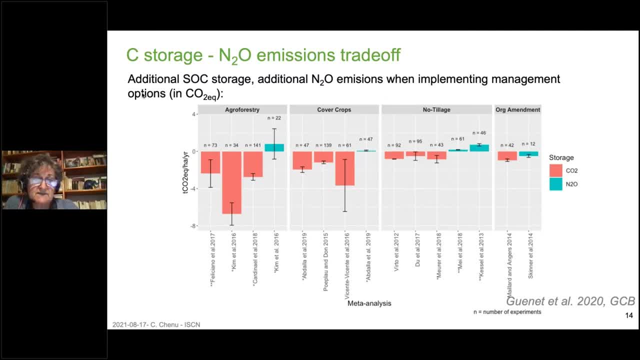 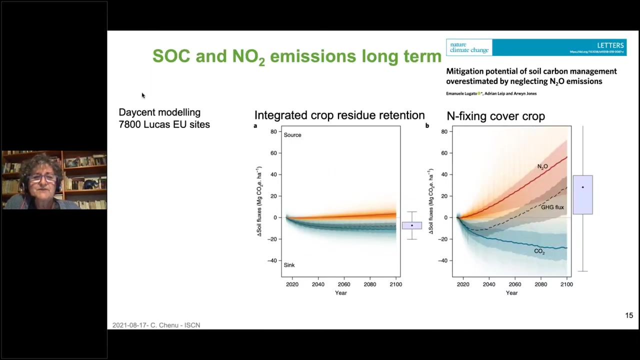 carbon sequestration but in some case nearly compensated, like again in no assembling, different metal analysis on no tillage. So it is necessary to establish a full carbon balance when implementing new management options. in order to estimate what is the net balance of greenhouse gases- And this it is also very important to consider not only the short-term, but 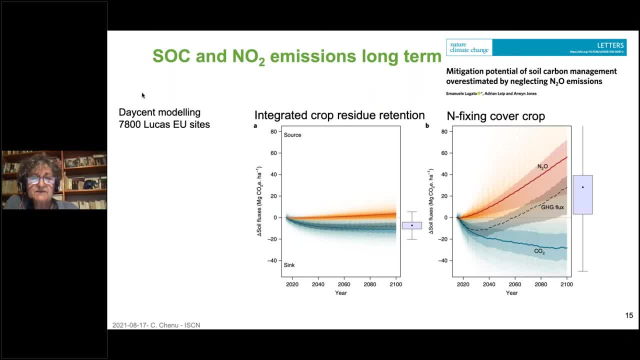 also the long-term. This paper by Lugato really brought, yes, information that is kind of provocative. well, it makes you think. They measured using, well, they model- excuse me, using DASENT. so a biogeochemical model, the model, the. 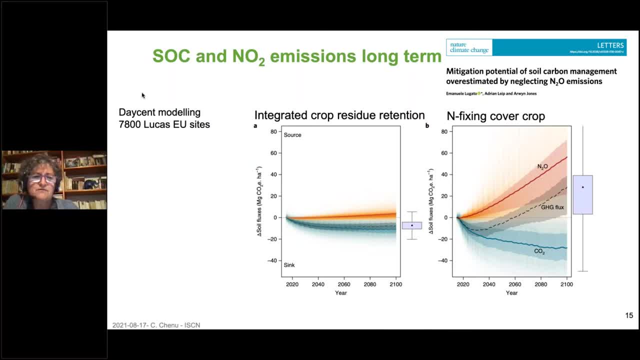 effect of two, of the implementation of two different management options on carbon storage and on N2O emissions, And they did that on the nearly 8,000 sites of the LUCAS. LUCAS is the sole European, sole monitoring system So wide. diversity of pediclimatic conditions. The two management options that compared, compared to the baseline, were integrated crop residue retention with reduced tillage And were implementing a cover crop between successive cash crops as as soon as they were more than two months between two successive crops. 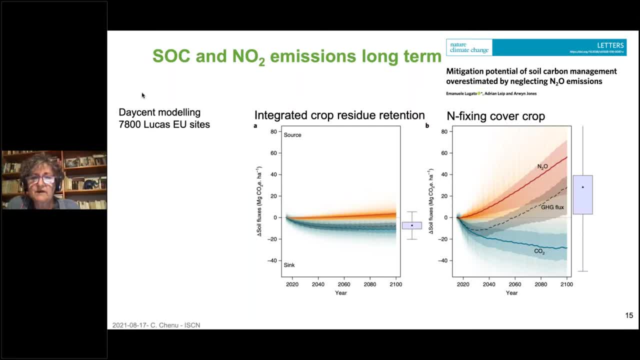 And this cover crop was a legume, N-fixing one, What you can see. so the graphs represent carbon storage. So this is here in green and it is negative uptake and N2 emissions in red and appear as positive. What you can observe. 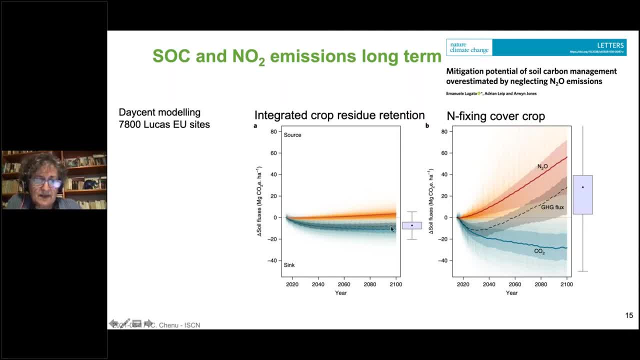 for the integrated crop. residue retention is a small effect on carbon stocks that plateaus around 2050 and a small but continuous increase of N2 emissions. At the start, there's low N2 emissions because the nitrogen is assimilated by the microbial biomass. 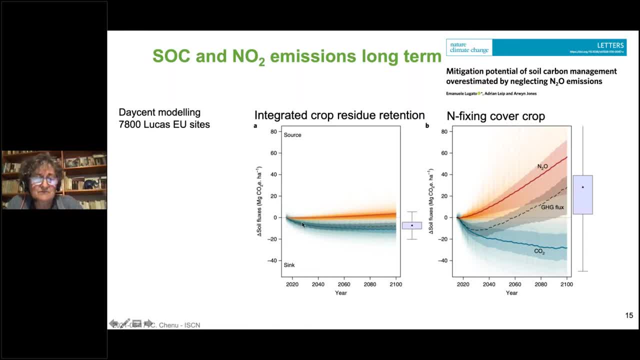 that is, decomposing the additional residues added to soil, And after it steadily increases, the balance remains in the negative zone, So it's favorable. Now if you look at the scenario with the N-fixing crop, you see that the carbon storage is much higher. 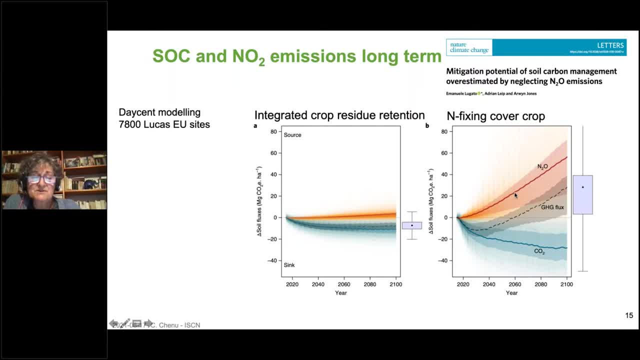 and it also plateaus, but N2 emissions they never plateau, They never plateau. And the result here is: after in their simulation, after 2060, there's a net emission of greenhouse gases in this system. So this I think it's kind of it's really. 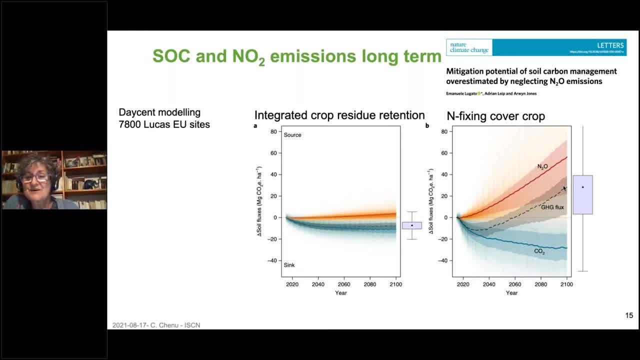 it's really stimulating to devise cropping systems where well to think differently the different timescales, and to devise cropping systems where N2 emissions will not offset the carbon storage. Well, in that in their simulation the mineral fertilization was adjusted to 70%. 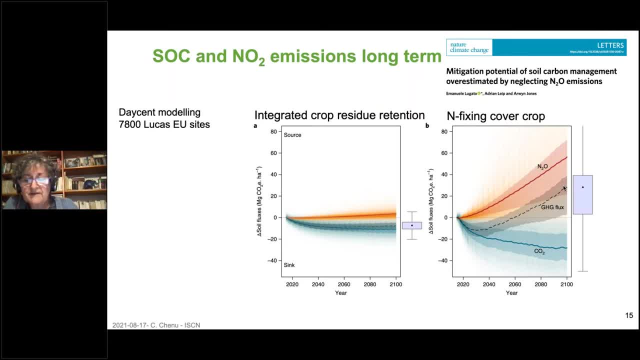 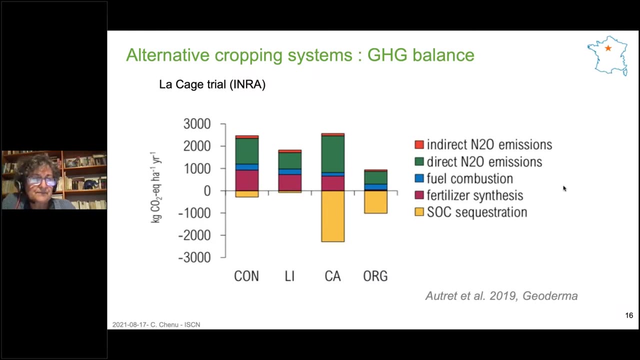 75% of the fixed N by the legume. So there was some mineral fertilization. Okay, So think about the time And again. let's go back to the case study of this comparison between alternative agroecological system in cerealic culture. 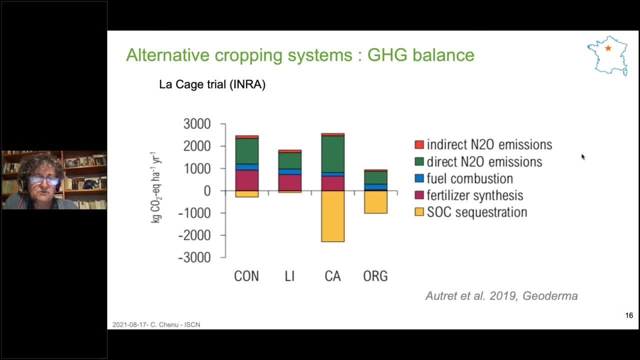 What Benedict Dautrey did. also is she what I showed you already. she quantified organic carbon sequestration. It's here in yellow. She quantified, she measured direct N2 emissions, but she also quantified through the leached nitrogen. 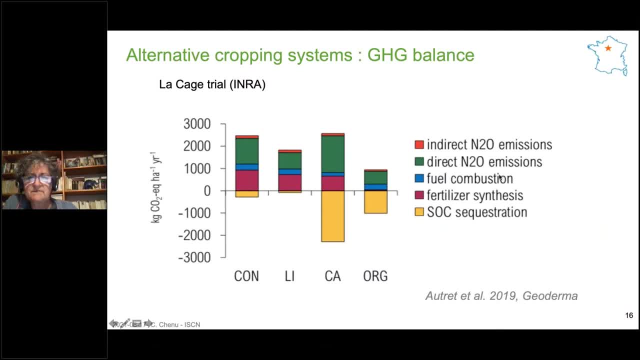 the indirect N2 emissions that do not vary much among the system. She quantified, she assessed fuel combustion in the different cropping system and the cost in terms of greenhouse gases of the fertilizer- synthetic fertilizer- used. You can see that in the conservation agricultural system. 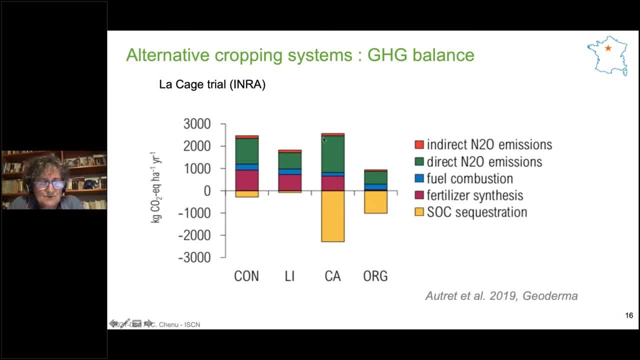 the other greenhouse gas emissions related to the cropping system and the other greenhouse gas emissions related to the cropping system. So this is kind of disappointing and it's nearly the same situation in the organic system. This is kind of disappointing to have a nil effect at the end. 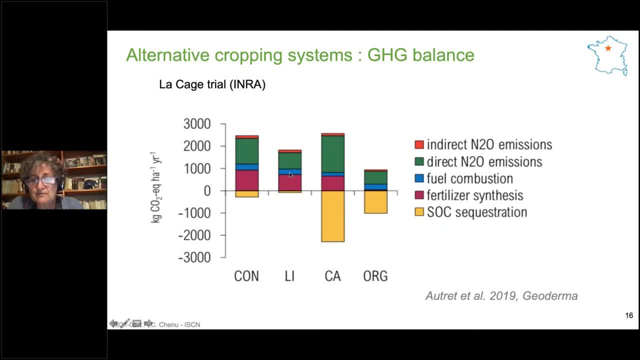 But if you compare to the conventional and to the low input system, these are net emitters. Here you have zero net emission and here you have systems that are net emitters. So it's necessary to measure to establish the greenhouse gas emissions. 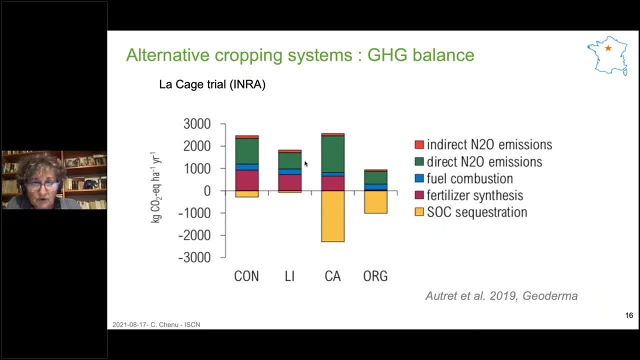 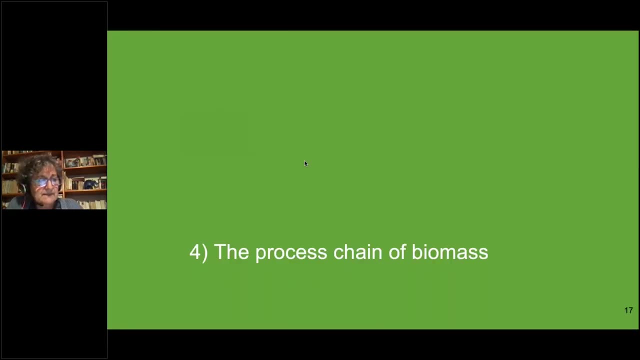 So it's necessary to establish the greenhouse gas balance between carbon and N2O, To consider the different operations in the cropping system, to integrate different and different durations and to consider the long term effects as well. And the last example and point I would like to raise: 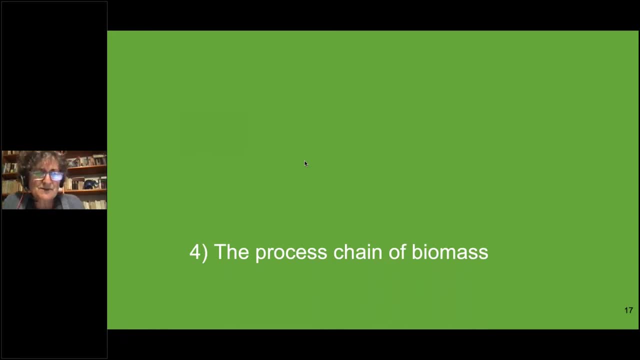 where I do not have strong statements to make, but it corresponds to questions that we repeatedly have from farmers in France and from actors of the European Union and from the leaders of the food chain. They ask what is best: Should they return to the soil the residues or the composted residues? 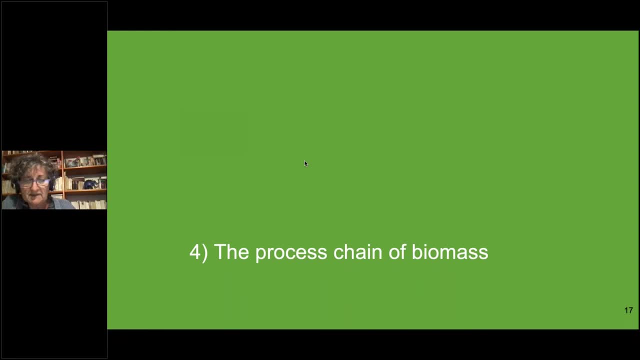 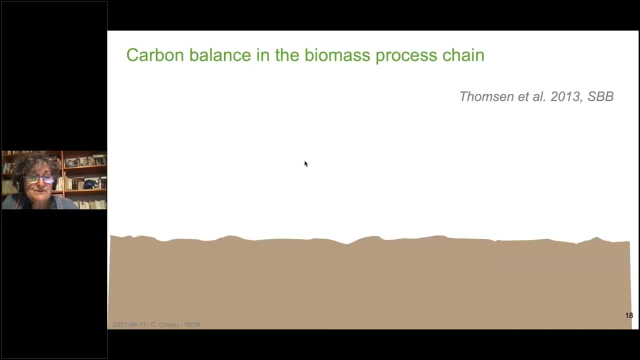 or the digested after some methanization, or even the pyrolysis, And actually there is nearly no study. I just was able to find one study quantifying the balance of carbon and N2O, and actually there is nearly no study. I just was able to find one study quantifying the balance of carbon and N2O. 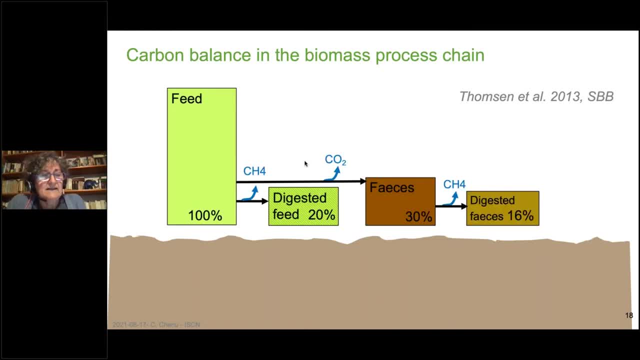 over the biomass process chain. so they measured Thompson it also Danish colleagues, they measured the mid measurements so they were able to establish the balance that for one given amount of carbon in the feed, 100%. they applied it to soil also. the digested feed, so digested, only remained. 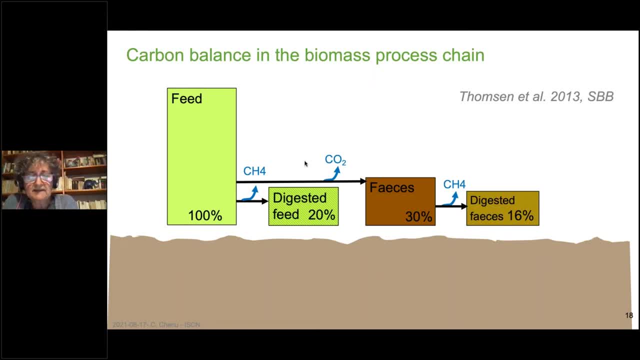 20% of that, the faces of the animals that had consumed the feed, and this corresponded to 30% of the initial carbon. by in the biomass or the digested faces, these correspond to 16% of the initial carbon in the biomass because, of course, there had been losses by respiration and by myth. 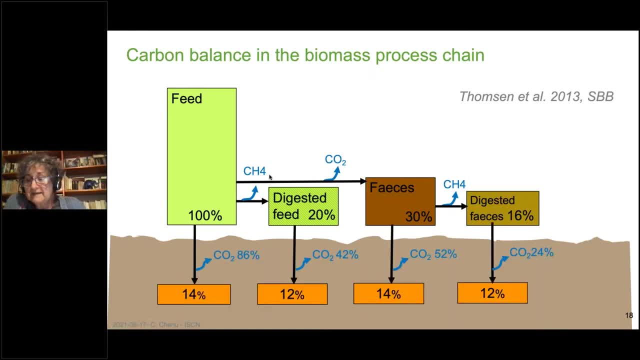 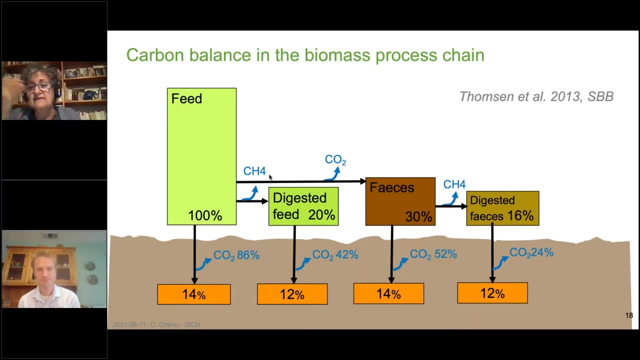 as methane, and they measured the balance in soil, what remained after two years after applying these two, 120 and 30 and 16 percent of the initial feed, and they actually found that there was not much differences in terms of salt carbon that were stored. So again, this is the only study we could find. I could find. 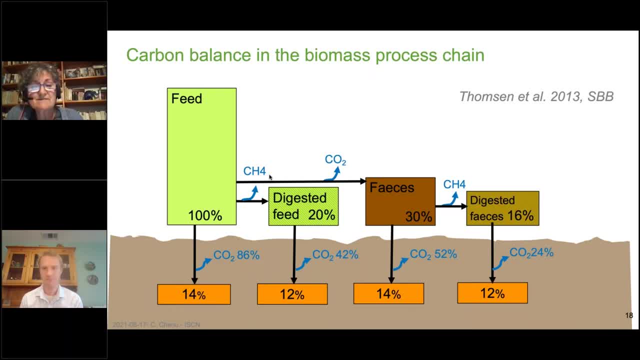 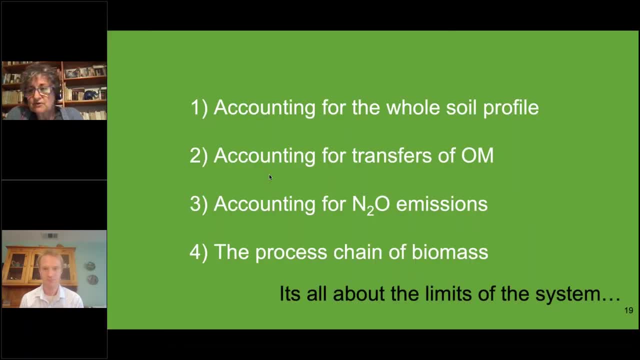 So this is likely to be variable among conditions, but I think this is a very important question, that more studies are needed there. So now to conclude, I just have two more slides. In fact, when does increased organic carbon storage yield net removal of greenhouse gases? 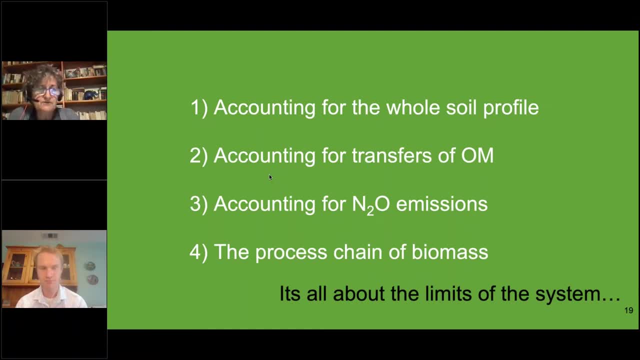 For that. it's all about limits of the system, accounting for the whole soil profile, accounting for lateral transfers of organic matter, accounting for N2O emissions in the system from the soil and in the cropping system, and accounting for the balance of carbon nitrogen nitrogen. 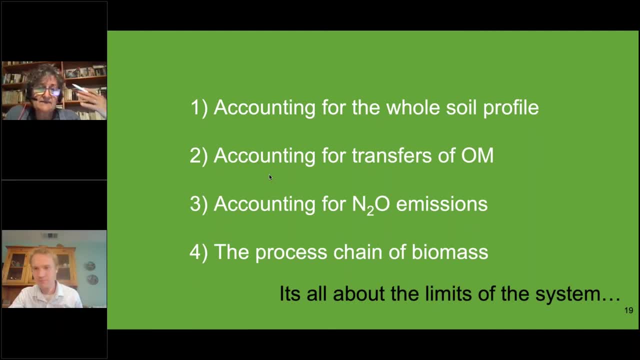 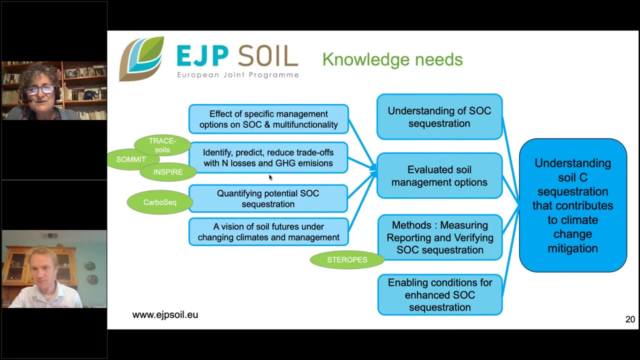 nitrogen in the process chain of the biomass, And there are, for that, well, a number of research. needs Well, to give you one image of what we're doing, I'm coordinating a European joint program- the joint program soil- that assembles or participate 24 institutes from 24 European countries. 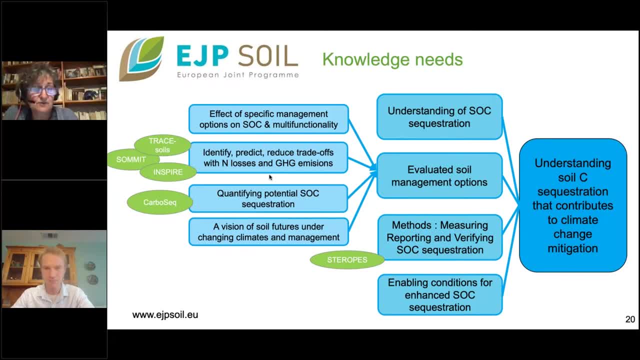 And we have different expected impacts and we have defined the knowledge needs. One of our expected impact is The understanding of soil carbon sequestration that contributes to climate change mitigation- Exactly the topic of the webinar today- And we identified that we had four categories of question. 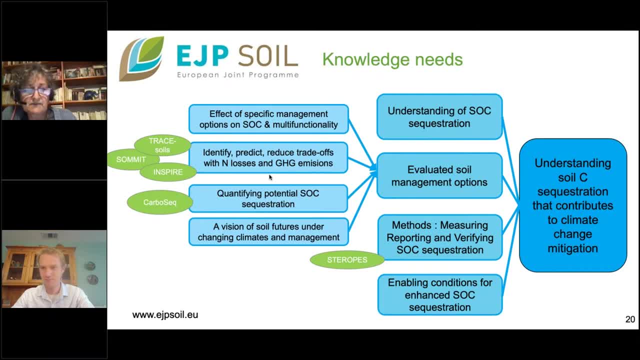 We needed to improve knowledge, needs to improve understanding of soil organic carbon sequestration, and we will have calls on the role of soil biota, on the permanence of soil carbon, on saturation, on deep soil carbon, on soil geometry. 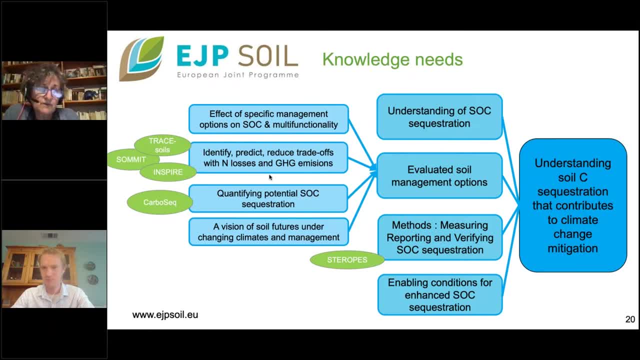 We need to evaluate soil management options And we We will focus. we are focusing on the effect of management options that allows compromises between soil, organic carbon and other functions expected from soils. We focus- and that's the topic of today- again on identifying, predicting and reducing tradeoffs. 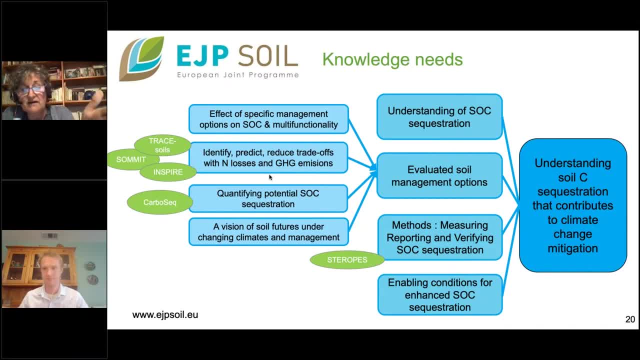 with nitrogen losses and greenhouse gas emissions. And so far we have three research projects already financed that are working: two on mineral soils and one on organic soils- very different organic soils And we want to quantify the potential. So organic carbon sequestration: we have one project doing that on 23 European countries. 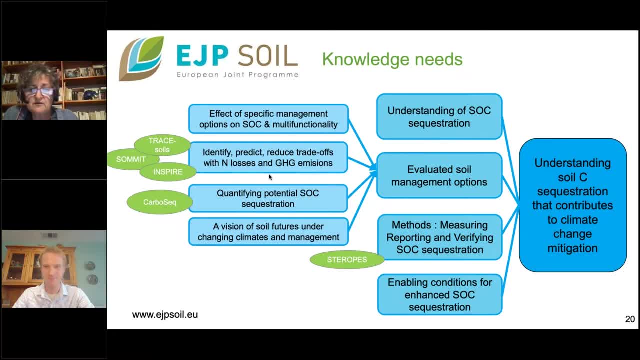 and we want to do scenario modeling. We think it's necessary to do scenario modeling with changes in policy, changes in climate, changes in consumer habits. What is also needed in terms of knowledge in this area is, of course, to develop measuring. 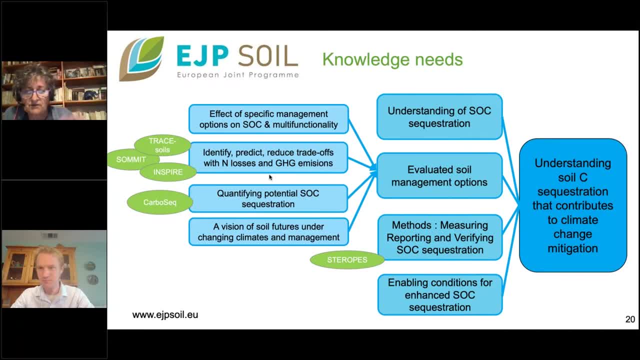 reporting and verifying soil organic carbon sequestration. So we work at present on remote sensing and we will work on proximal sensing And we do have yet projects on that, but we think that there are a lot of knowledge needs regarding the enabling conditions for enhanced soil organic carbon sequestration And on that. 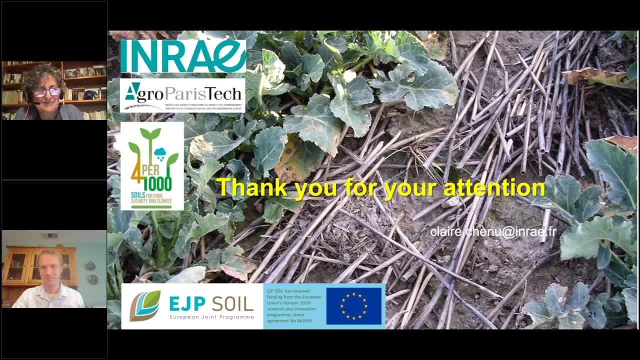 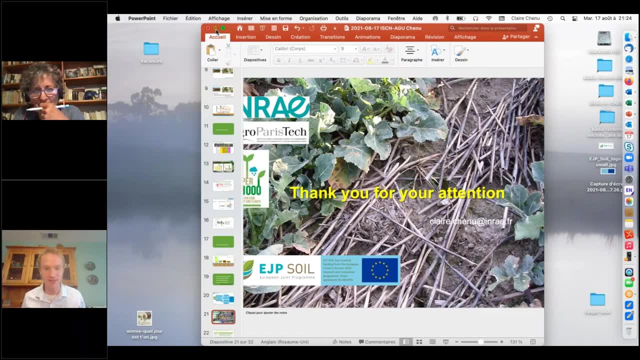 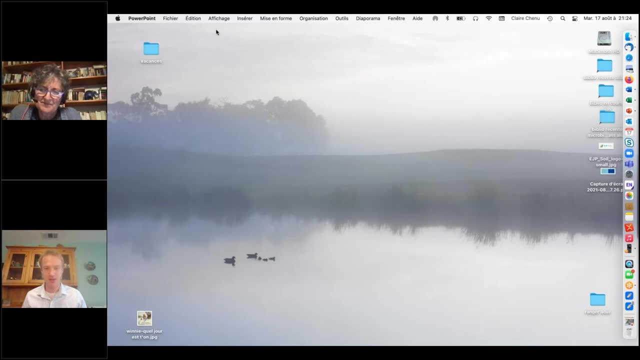 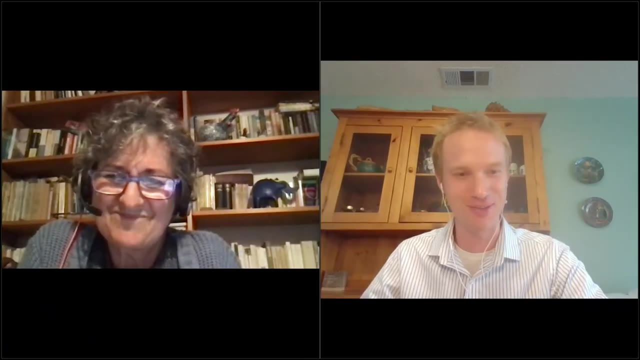 I would like to thank you for your attention Wonderful. Thank you very much, Claire. I think that was a terrific broad overview of the issues surrounding achieving net greenhouse gas removal in soil, and the case studies were really fascinating too. I now have some papers I have to go read clearly, So I'm going to address some. 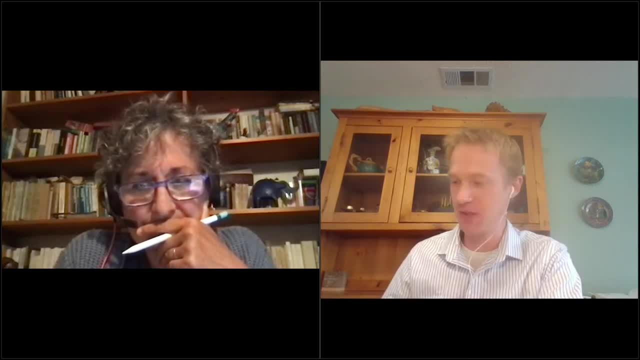 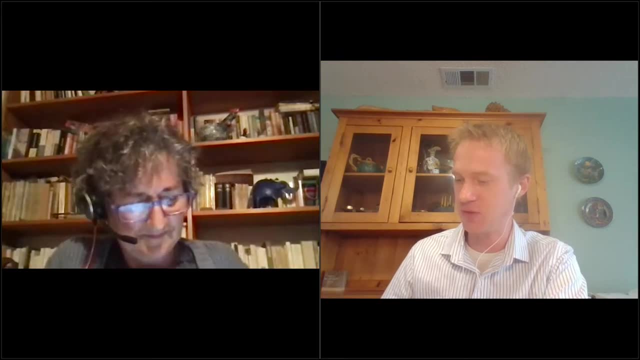 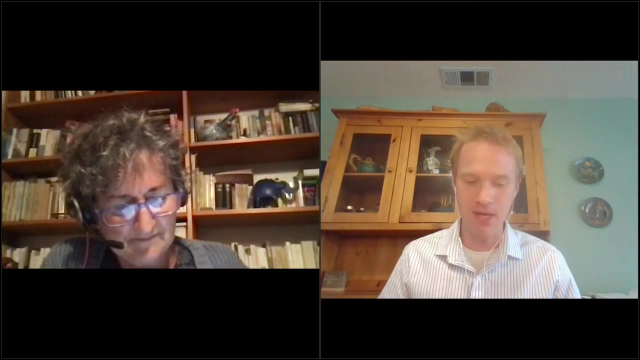 questions that came up from the audience today and then also that were submitted during the registration process, And one question that came up more than once that I think is an interesting one is how, apart from different management techniques that apply within an annual cropping system, how does shifting to more perennial land cover affect NTOO in particular, And do we know anything about this? Regarding NTOO, there has been, I think, especially into. well, it depends on the fertilization of the soil and then the soil is going to be covered, And so many of the areas in 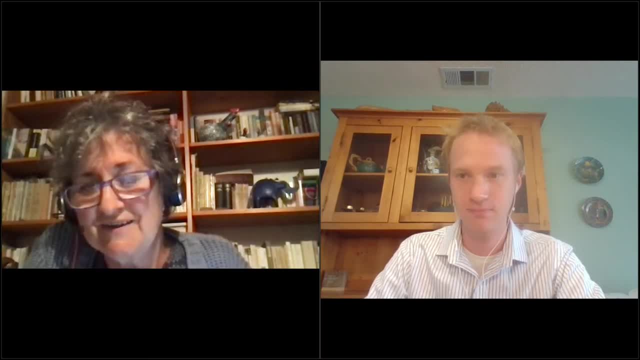 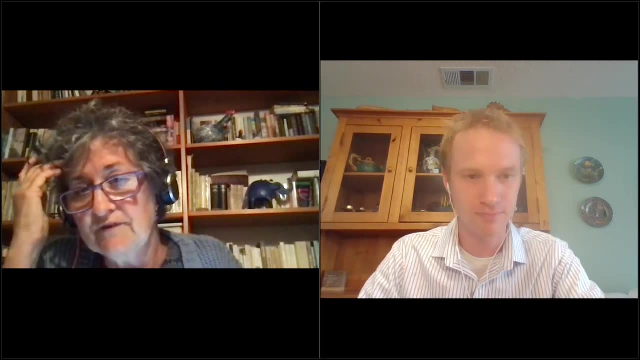 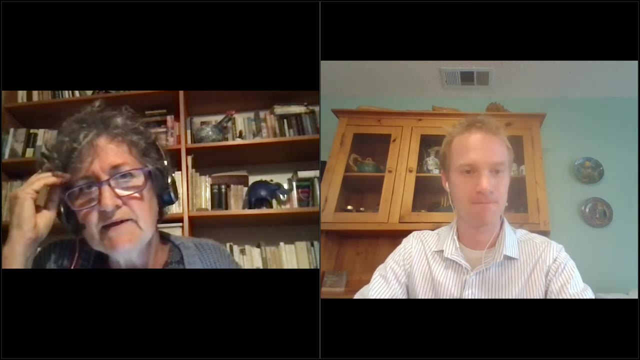 the soil we are talking about right now. we have, I think for the most part there has been a lot of your perennials. Well, the main factor of N2 emissions is the application of nitrogen fertilization to soils. I'm thinking of agroforestry. There has been some estimates. 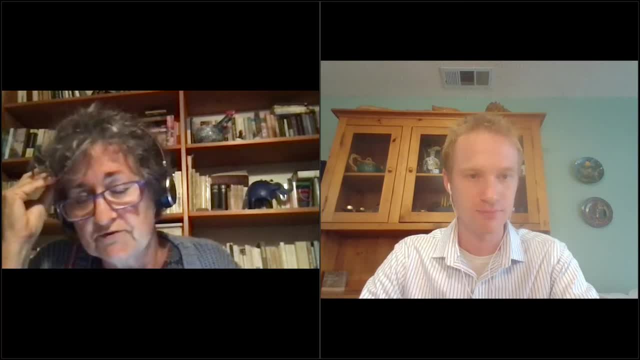 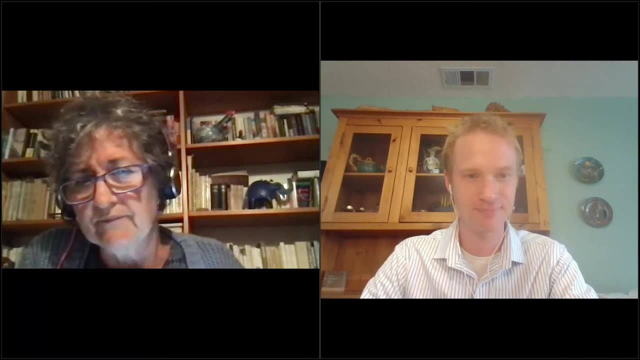 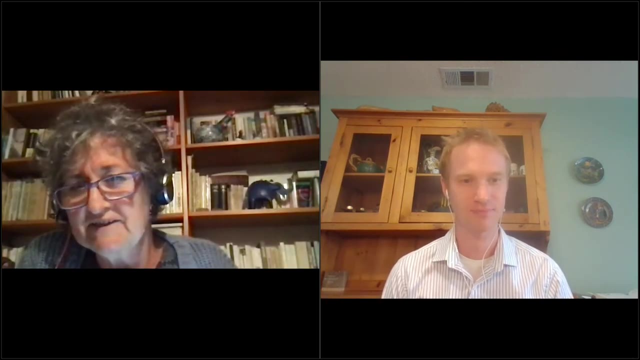 of N2 emissions from agroforestry. In general it is reduced compared to the counterpart. Well, there's no additional N2 emissions because of course the trees uptake the soil nitrogen and they can uptake it even from very deep soil layers. Quite often also, soils are drier, so 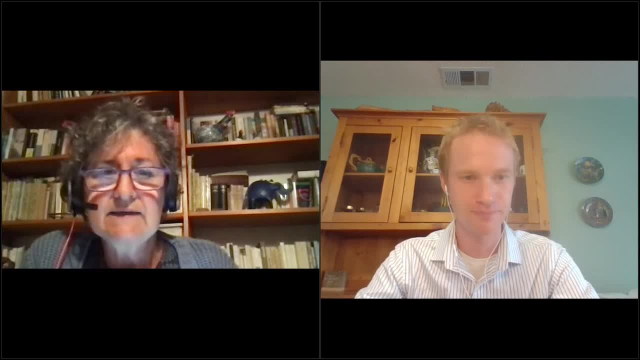 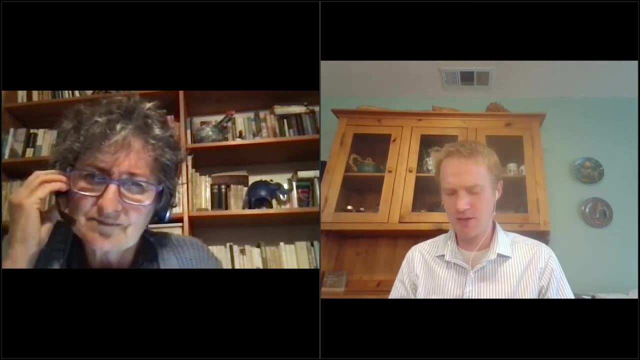 conditions are not favorable for denitrification, But the only exception. there were some measurements with legume trees and in that case there could be additional N2 emissions Interesting. That makes sense. So another question that came up repeatedly in different forms that I think would be: 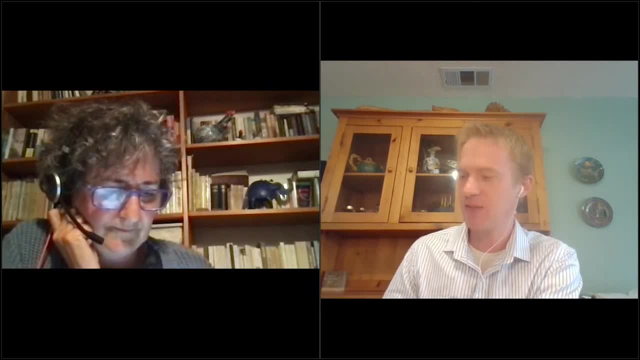 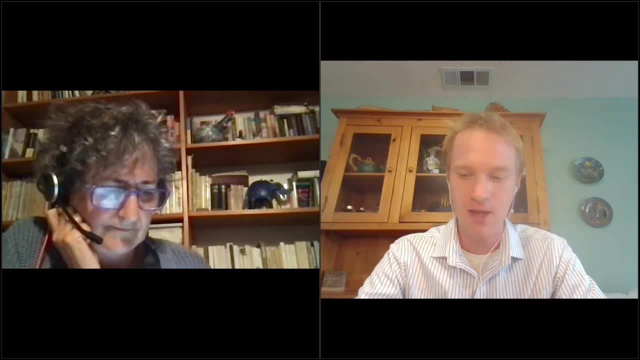 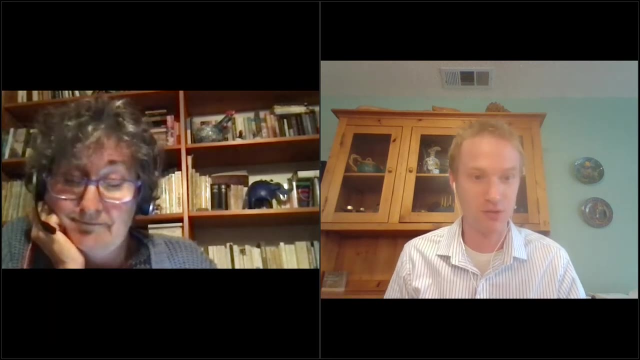 interesting to discuss is it relates to scaling, And so the field experiment that you were discussing involved this very, I imagine, very laborious set of chamber measurements to get N2O fluxes from one place, And then the modeling study covered vast areas. 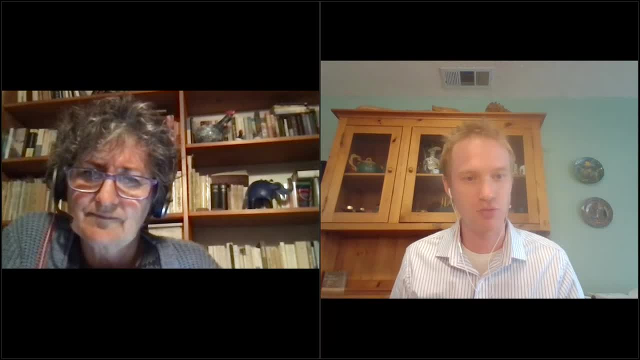 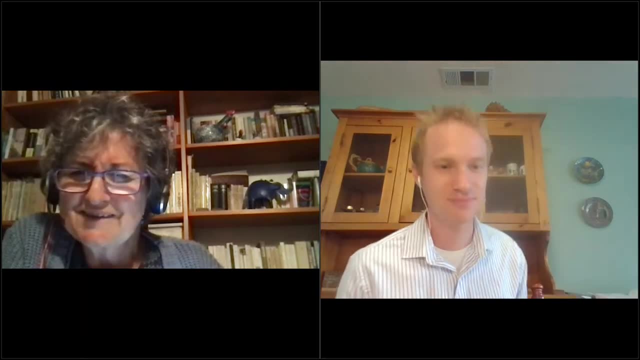 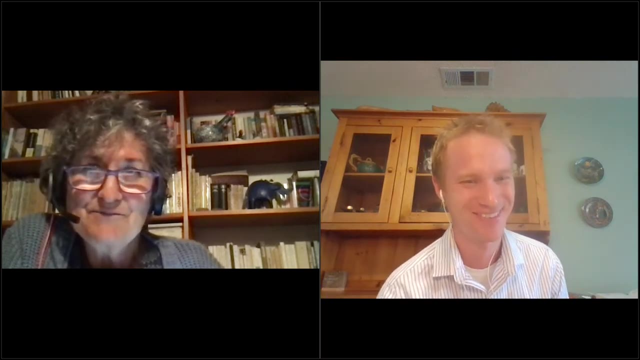 What do you think The right balances of those sorts of approaches for doing large scale monitoring of greenhouse gas emissions? Difficult question, Right? Well, I think the right answer, but I'd still like to hear your thoughts on it. Well, and I think- but you gave partly the answer- that we need to combine case studies. 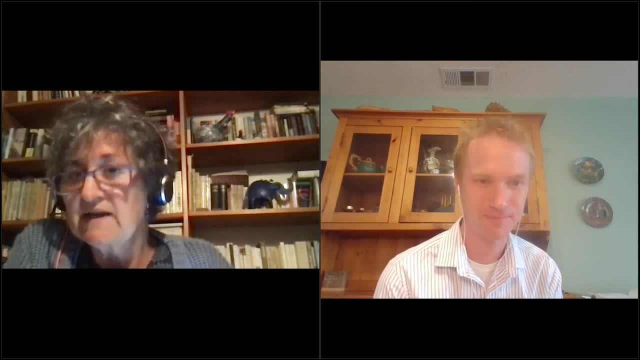 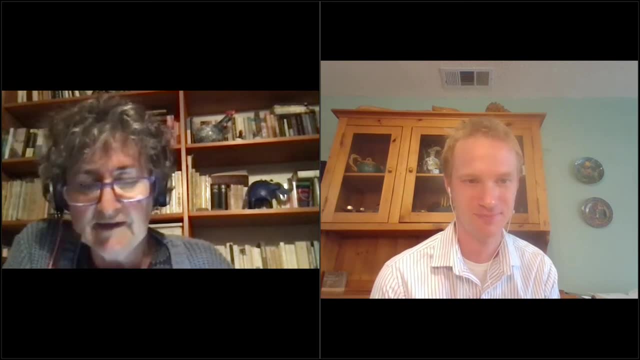 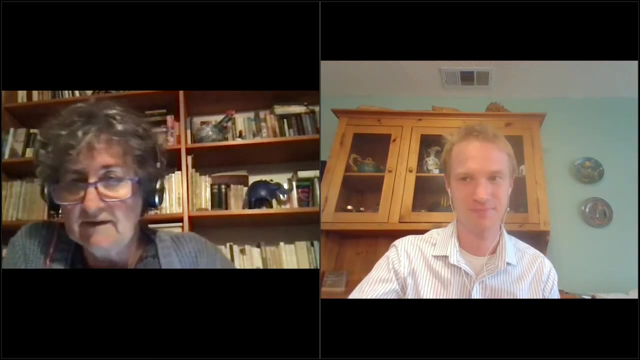 monitoring systems, and it's an issue to establish monitoring systems where, not only where, diverse measurements are made over time. These monitoring systems can be at long-term, coupled with long-term experiments, or just sites that are taken along a grid, like it is done in several countries, or at farmer's place. 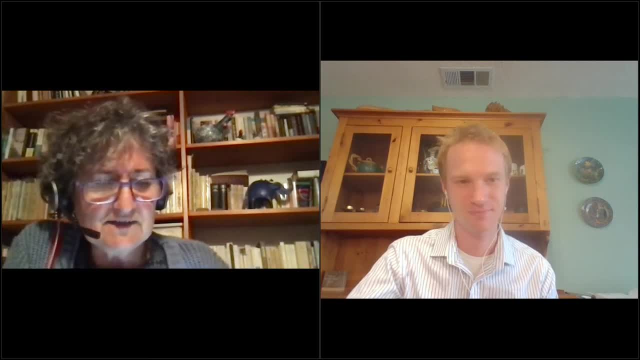 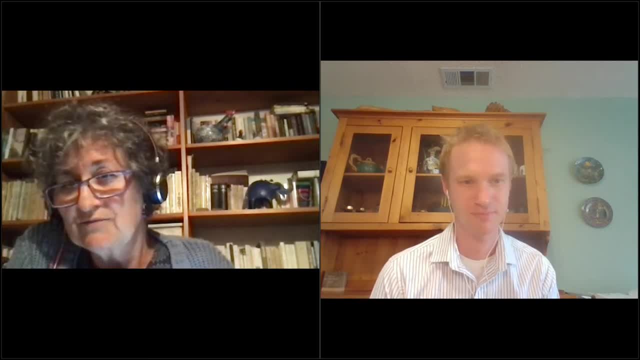 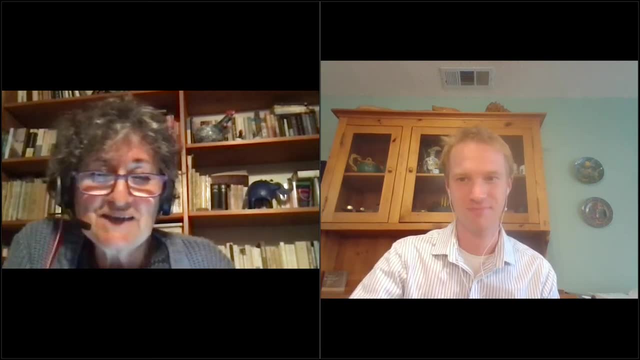 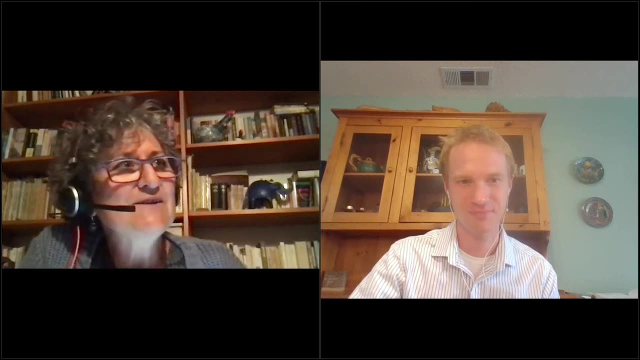 And modeling helps to change spatial scales and time scales. I think So. yes, I do not have a sorry, but I do not have the good answer to your question. Yes, One thing I'd like to say is that, as it's in another area, as an editor, 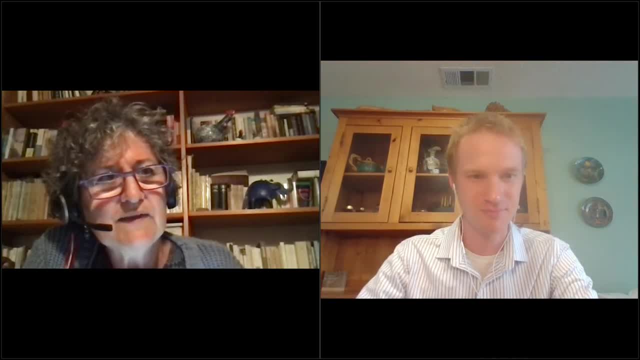 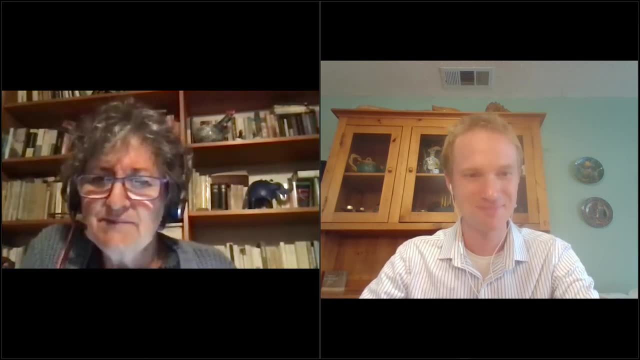 I am in a journal. I am amazed at how we tend to undervalue case studies. but to do a meta-analyze, we tend to undervalue case studies. But to do a meta-analyze you need case studies. To calibrate, to validate a model, you need case studies. 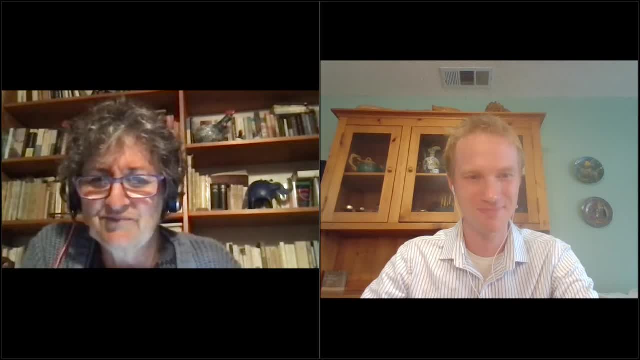 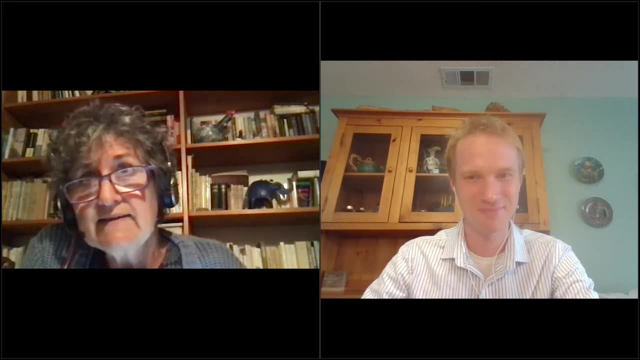 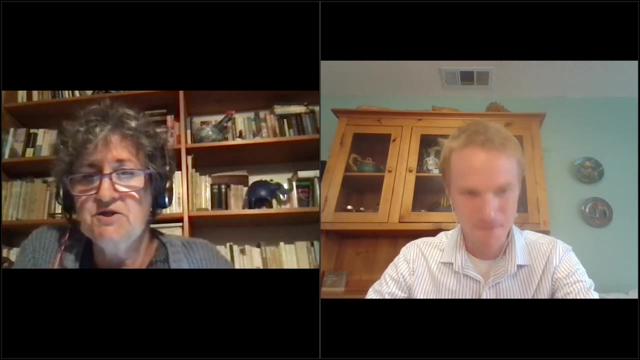 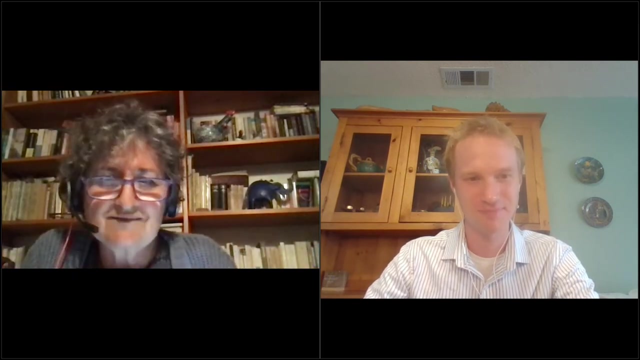 So, even though as scientists we tend to undervalue case studies, we absolutely need them, but maybe we need to set them in a more coordinated way, that is, along a framework. Where do we lack information for which, you know, pedoclimatic versus management conditions do 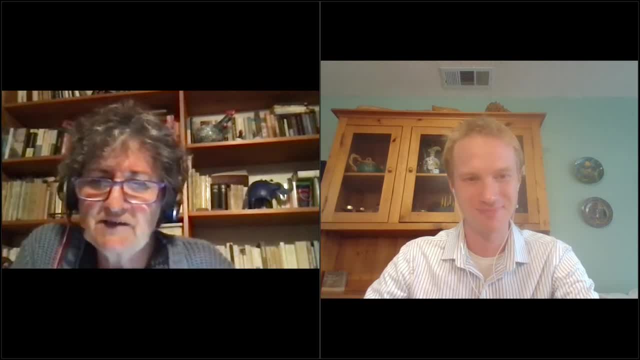 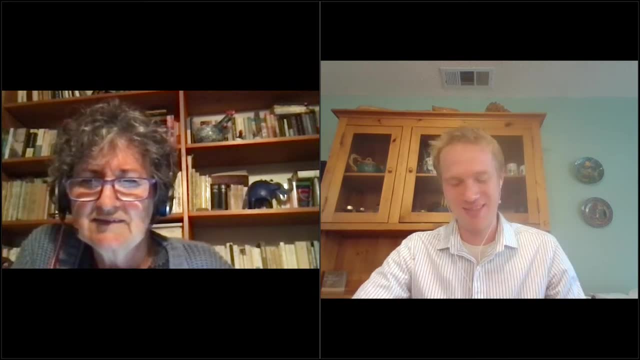 are: do we lack information? So maybe the effort should be done in that direction. Yeah, that's a very good thought. Thank you for that insight. I think that's that's important for everyone to remember, because we tend to, we tend to focus, we tend to go to the. 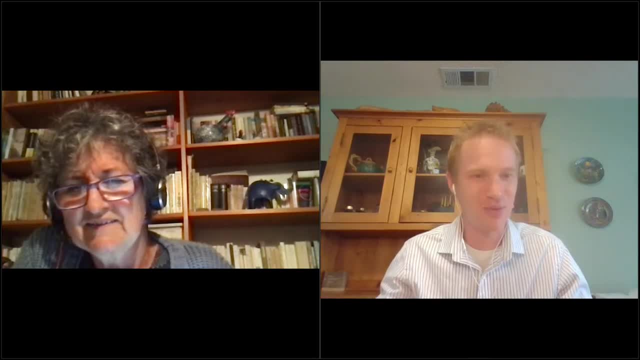 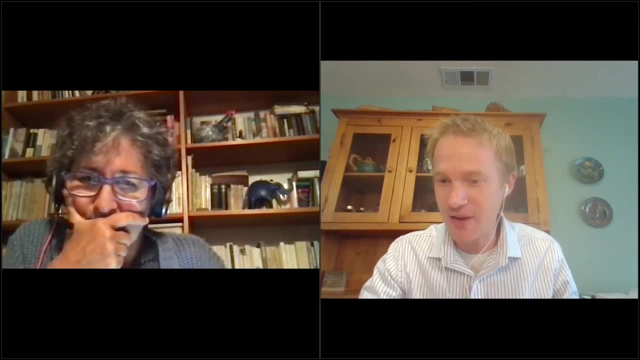 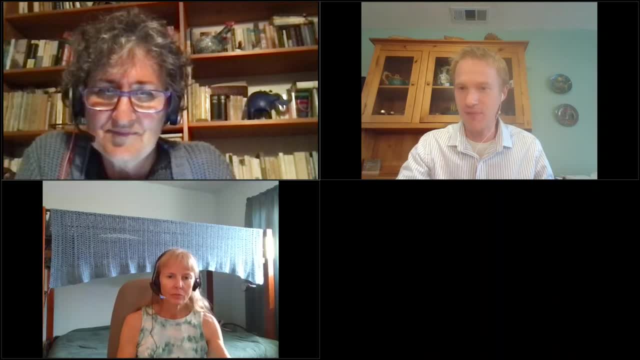 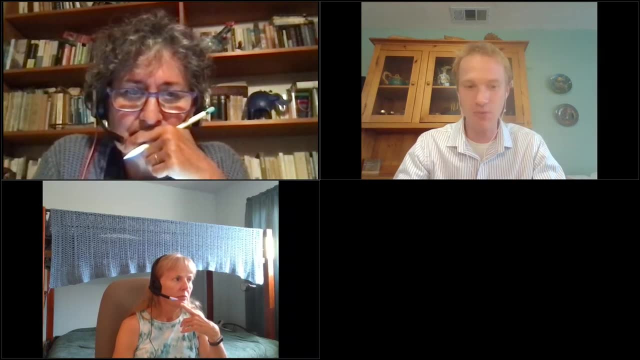 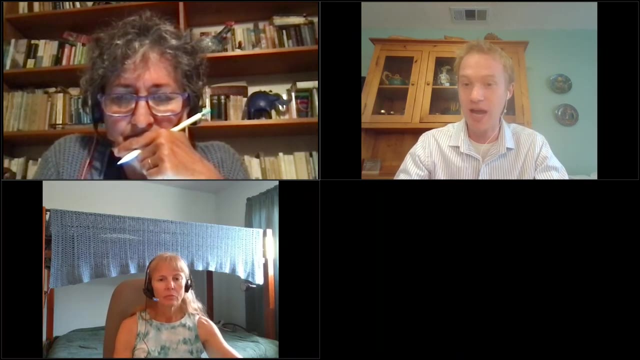 And before we do, I forgot to mention something at the start. Firstly, feel free to post questions at any time in the questions feature, but I should also mention that we have a discussion forum we've set up on the ISCN website via this Padlet platform, And so if you go to the chat, 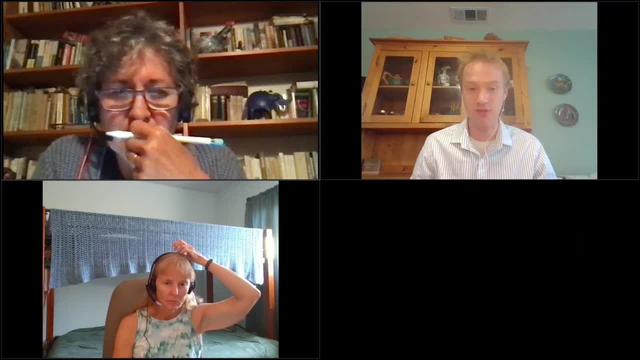 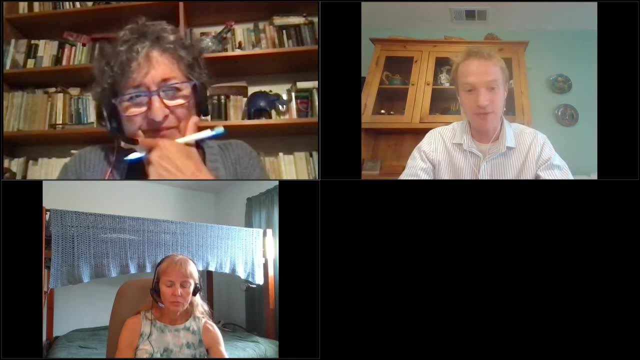 then attendees are welcome to to post further questions and discuss things amongst amongst themselves on the Padlet, even after the webinar is done. So take a look at that if you're interested in continuing the discussion And without further ado, we'll we'll move on to. 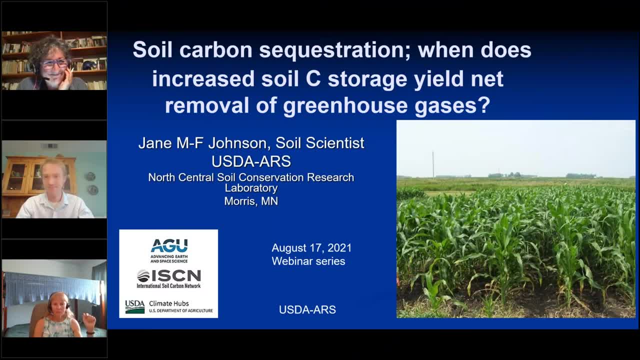 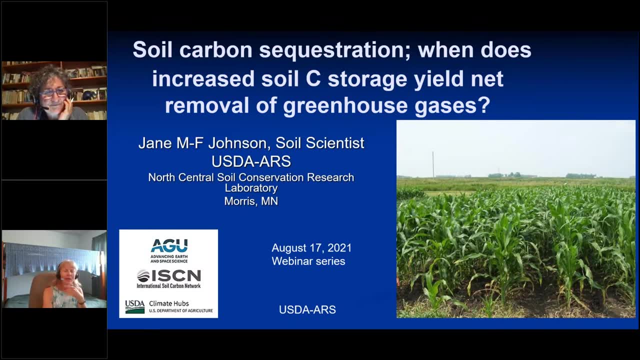 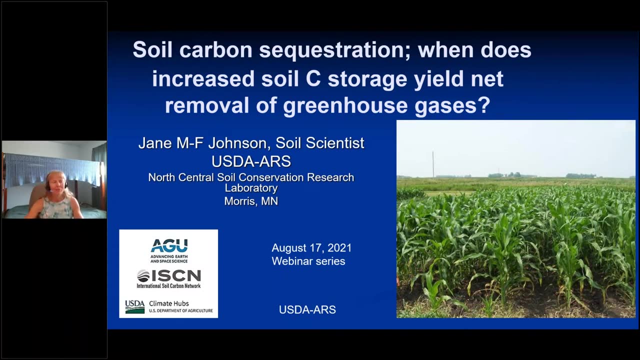 hearing Jane Johnson. Thank you, Eric. Want to give me a. I think things are working, So, if not, somebody please let me know. Claire, you did, Claire, you did a fabulous job of setting me up. I think our talks are going to compliment very well. Again, I'm Jane Johnson, I'm a the research leader and a research 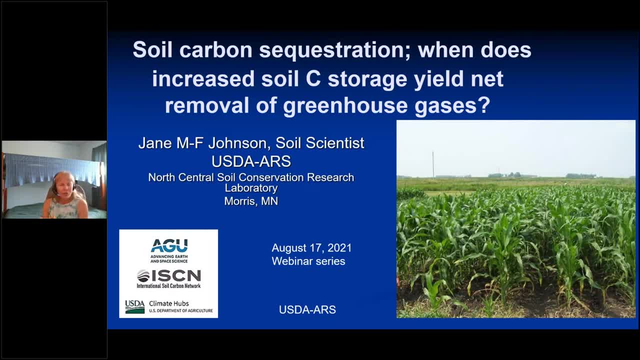 scientist with USDA ARS in Morse, Minnesota. This is a corn soybean system that is primarily- you know we're at the in the middle of the well, not the middle of the corn belt, but certainly part of the corn belt- 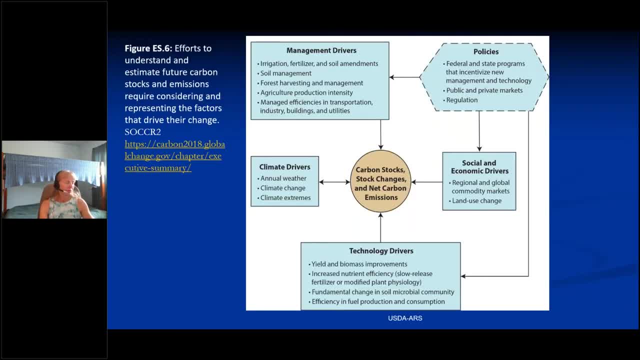 And so Claire set us up very nicely And if we think about this question and we're trying to get at the how to answer this idea of of the carbon stocks, how are the carbon stocks changing And how do we look at that in terms of net carbon emissions? And that has to include 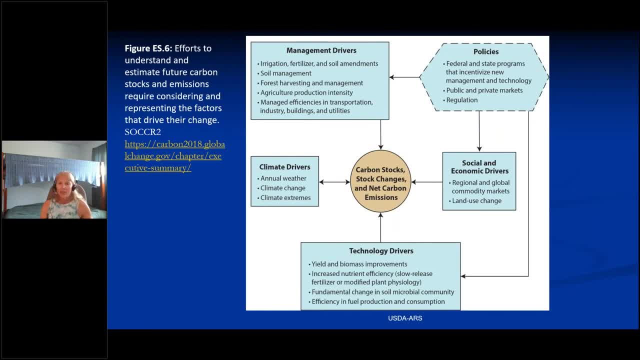 the other greenhouse gases, particularly nitrous oxide, And if you're in animal systems, then it also becomes important to be looking at methane as well. So this is out of the recent, fairly recent- state of the carbon cycle report that came out in 2018.. 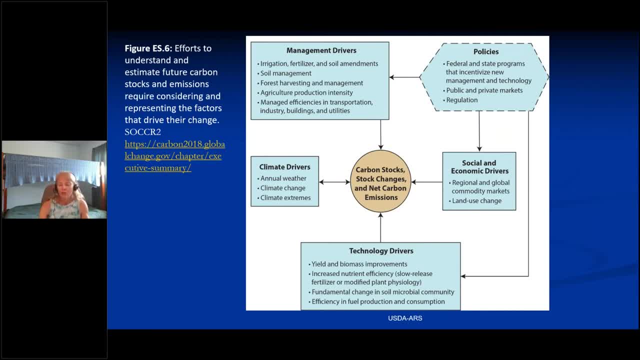 And really this kind of drives home, the importance of, of looking at the fact that there's management drivers from agriculture that could be soil amendments- Claire did a nice job of talking about lateral movement when you use manures or other things. Soil management, tillage, et cetera, The production intensity. So these are all. 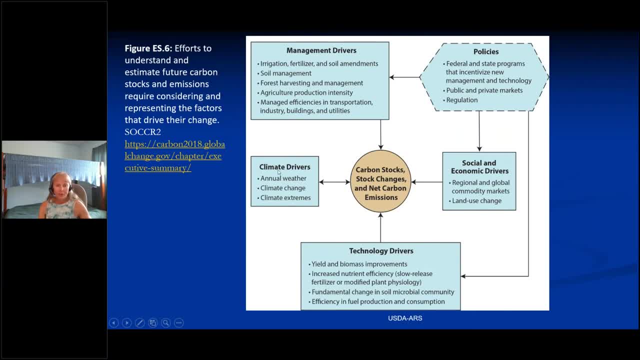 important management drivers. They interact then with the climate change, annual weather, the extremes. those are all going to have a role on these dynamic processes. Also, looking at technology drivers: Are we improving our ability to look at nutrient efficiency, whether it's slow release fertilizers- are they actually changing? 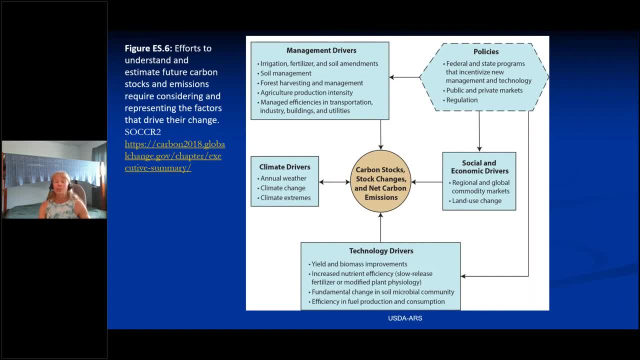 The amount of nitrous oxide that comes off, or do they just simply change the timing And then the role of the microbial community? The soil microbiome is a huge area of research, from a vast variety of research questions And then looking at production, et cetera. 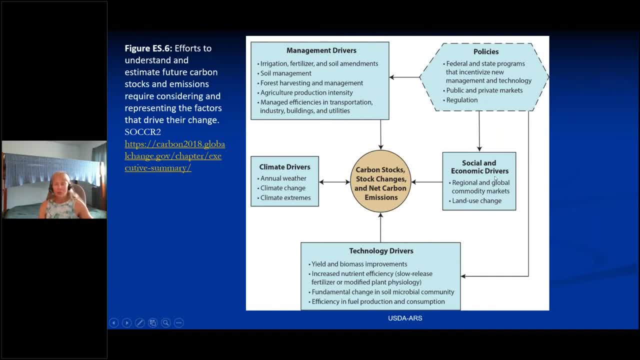 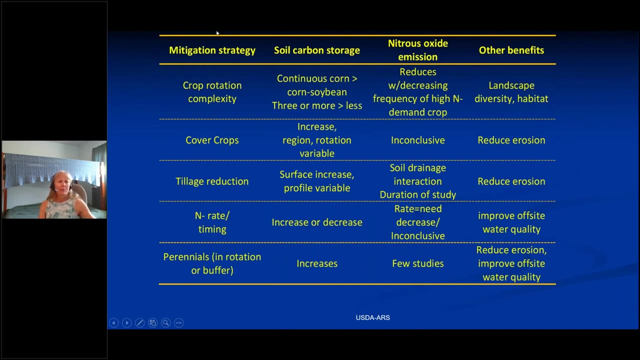 Also overlaying this is policy, and then the social and economic drivers, which are well beyond my expertise, but they certainly have an important role to play, to play as well as we move forward. So if we think about some of the mitigation strategies that, from a farming community, you may have at your disposal, you have 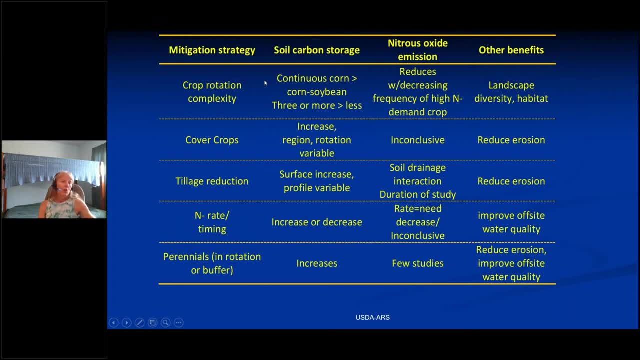 things like crop rotation and complexity, going from continuous corn all the way up to very long rotations that may be seven or eight years in length, And what they might do with nitrous oxide and that can be. they might reduce or decrease the frequency of high demand crops, which could reduce the amount of 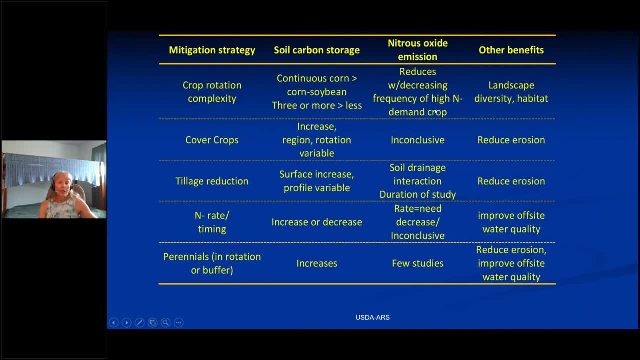 nitrous oxide and provide additional benefits. But again, you have to go in and look at it very carefully, just as Claire had shown in her studies. Cover crops: part of it depends on what are the cover crops. Are they legumes, Are they? 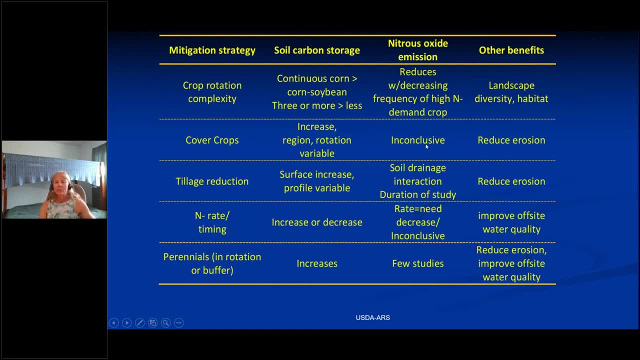 winter kill, et cetera, et cetera, And there's a limited number of studies that have really dug into the effect of cover crops. that may be going on. You have tillage and Claire did a wonderful job of showing you know some of the 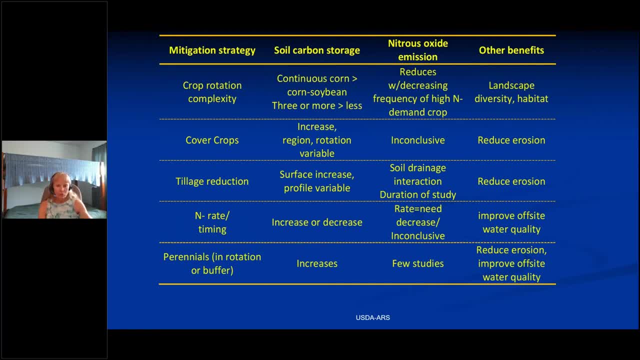 issues with tillage is that you have to make sure that you're not just redistributing it, And it changes the microclimate and changes the growing conditions that may be happening there. So it's important to understand what's really going on there and looking at least one increment below the greatest. 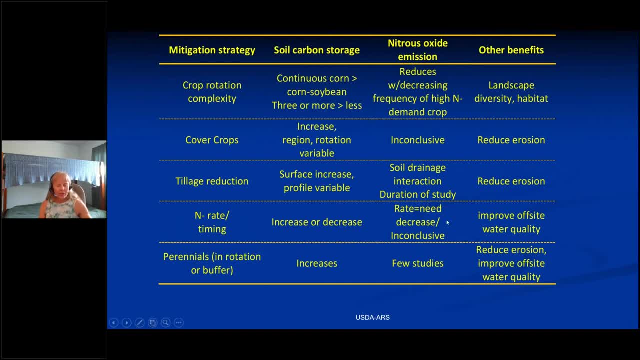 step the tillage and seeing what's really happening Over time and within those treatments the timing and nitrogen becomes important, And then also looking at perennials, And I'll give a couple case studies from some research that I've done in Morse that addresses some of 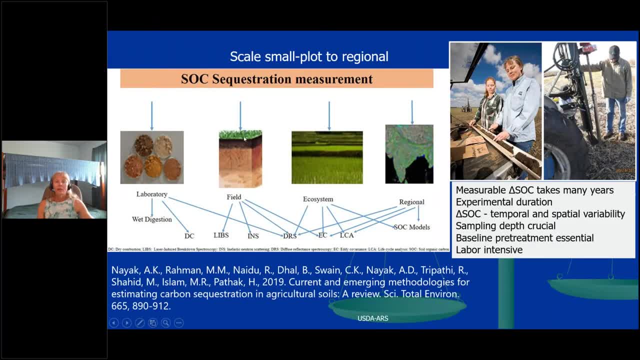 these options. The question came up about scale and that it depends on the question you're trying to answer. For one thing, are you trying to do national or regional accounting, Or are you trying to do national or regional accounting? Or are you trying to do national or regional accounting, Or are you? 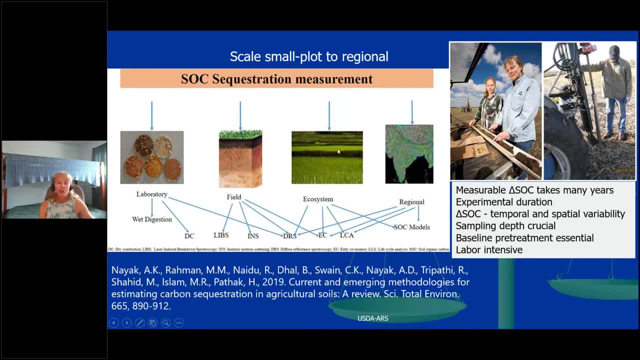 trying to answer something that's more specific at a regional or ecosystem. Most of the research I've done has been at the field scale, where we go out and we poke holes in the ground, we collect those soil samples, we take them back to the lab and we try to account for temporal and spatial variability, Both of 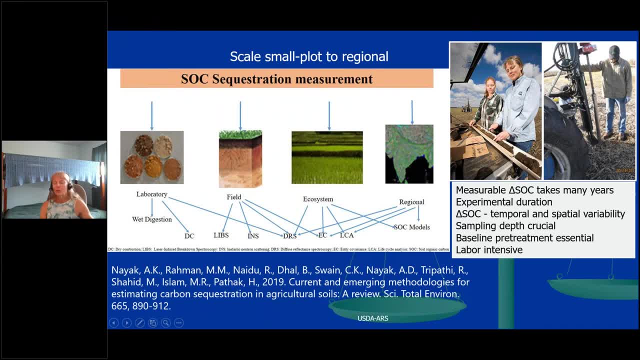 them are certainly can be an issue. You're looking for small changes against a large background. Knowing where you start is very important. I encourage you. if you're interested in methodology, there's a recent paper that came out by Nyack that does a very nice job of reviewing. 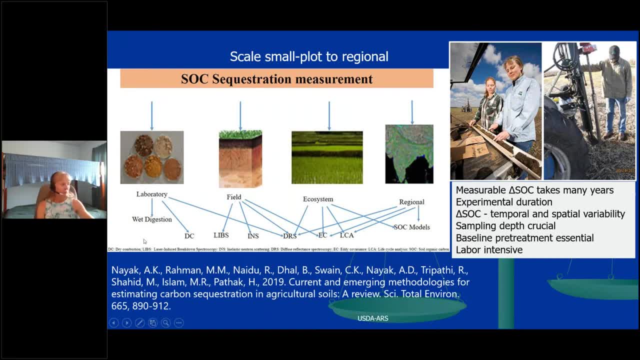 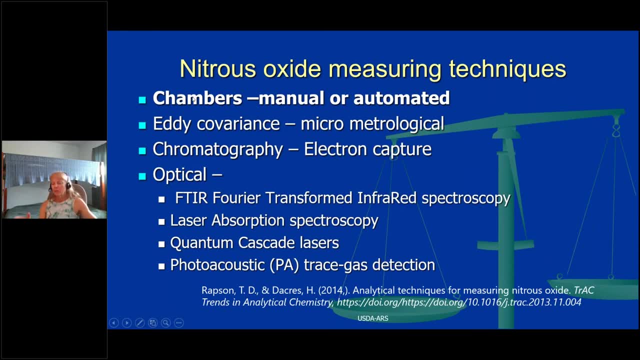 some of the options that may be available. Likewise with nitrous oxide. there's a variety of measuring techniques. Probably the one that has gotten the most leg reaches or the most papers put out are the simple chambers, closed vented chambers. it can be manual. 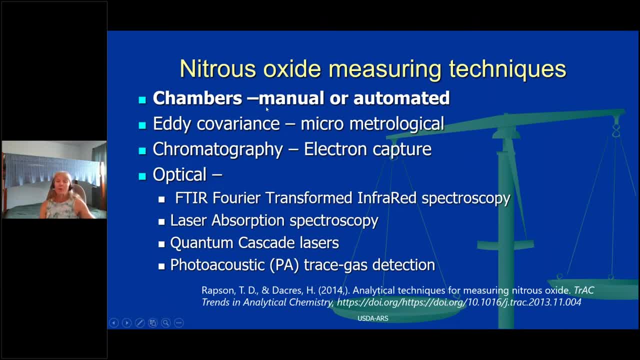 or automated. They have the advantage that you can put a lot of them out in the field to try to capture some of the spatial variability. They are hampered by temporal variability. If you use automated chambers you tend to get better temporal variability captured at the expense of 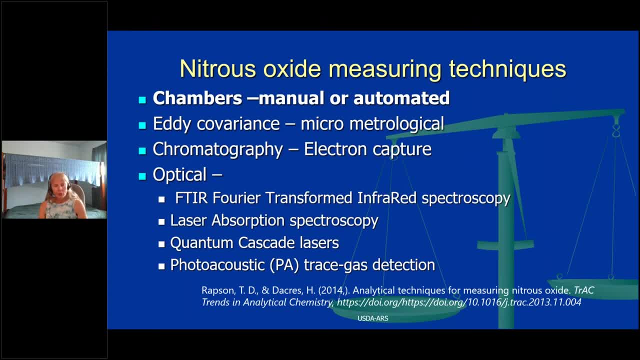 the spatial variability. There's new micrometeorological methods coming online Somewhere along the line. usually have electron capture as one of the tools for measuring by chromatography. There's some optical methods and again there's an analysis paper on the methods. 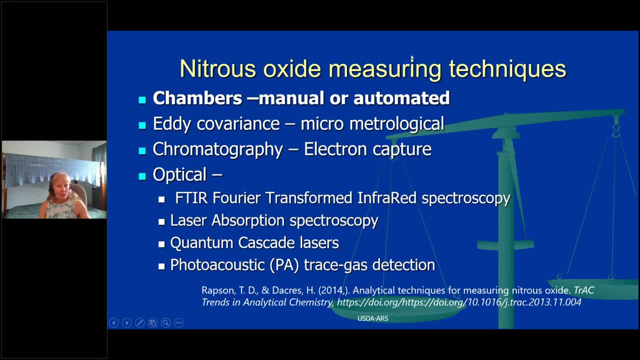 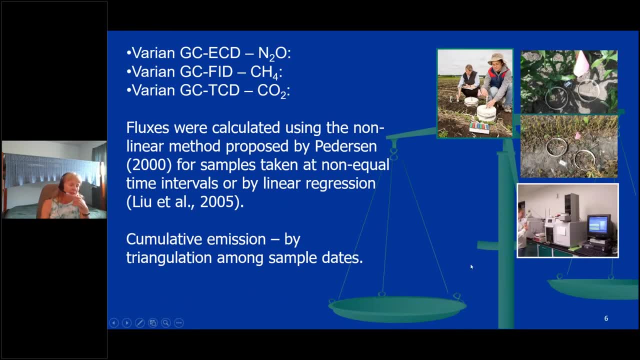 that came out in 2014.. I'd encourage, if this is a topic of interest, to check it out For the studies that we did in Morse. typically, we were going out and collecting. We'd pull a sample. We'd transfer that into a sample. We'd transfer that into a sample. We'd transfer that. 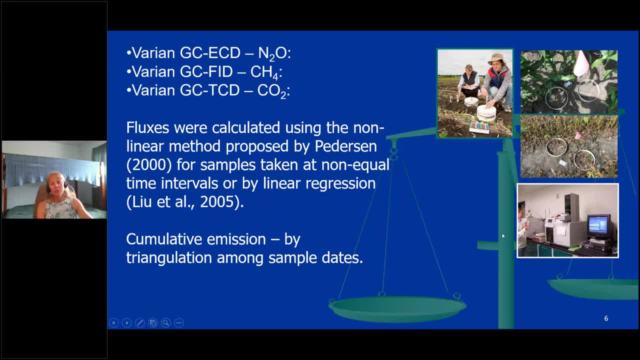 to a sample. We'd transfer that into a sample. We'd transfer that into a sample. We'd transfer that a vial. take it back to the laboratory. We measured these samples year-round. We'd go from planting to planting. Minnesota has very cold winters and we tend to get a pretty substantial spring flux of. 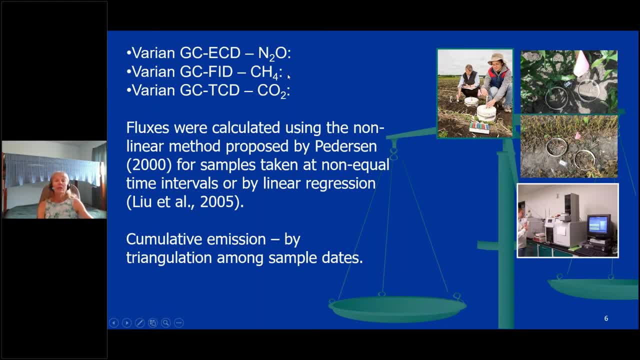 nitrous oxide that comes out. We did look at methane but in these row crop systems typically we've seen very little methane uptake or emission. They tended to be very close to backgrounds so typically we've neglected going out and measuring them. Like I said, if you were having 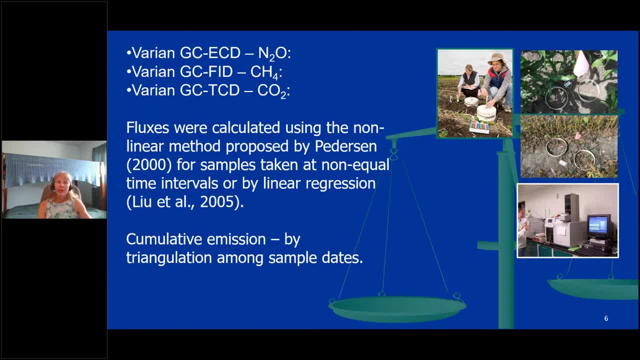 systems. where you're looking at livestock, then methane becomes way more important. or if you're looking at rice systems, for example, then you would have to pay more attention to the methane. We would go out, We would take repeated measures so we'd come back to the same spot. 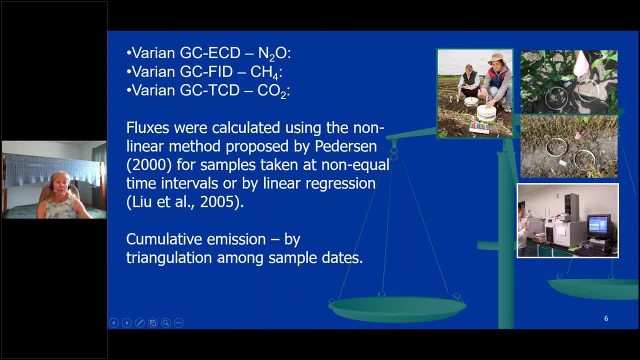 take another sample after these chambers were put on, calculate the flux and then integrate by triangulation among time to get our integrated point. Great job, I think, of capturing some spatial variability hampered by temporal variability Once you have the emissions. 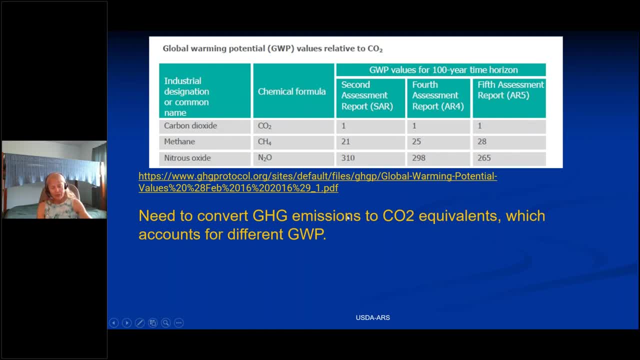 you can convert that then by CO2 equivalents, as was previously mentioned, to account for the global warming potential. The values there that are recommended have changed over time, and for nitrous oxide, typically they've reduced the value on a 100-year basis, but increased methane. 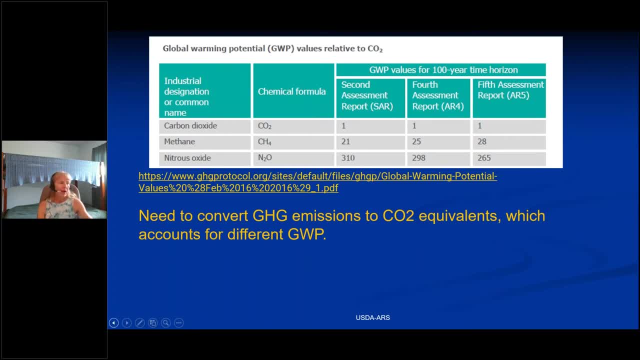 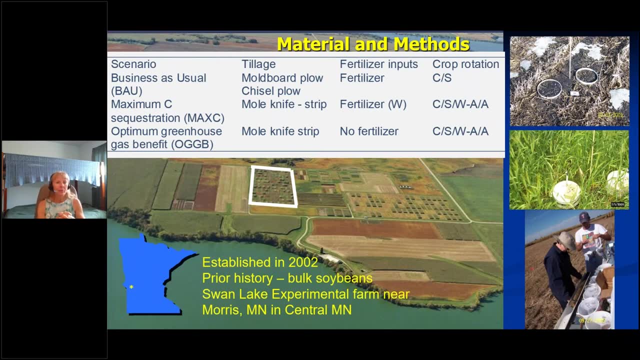 Nonetheless, you have to make that calculation if you're going to compare apples to apples. I'm going to transition and talk about just a couple of examples that we've looked at in Morse in terms of what has been some of the studies. These go back over the decade or so. 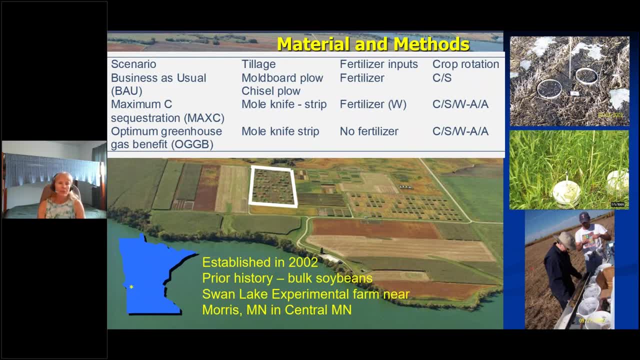 So one of the first studies that I did on nitrous oxide was part of a group effort referred to as GRACENET, which stands for Global Greenhouse Gas Reduction Through Agricultural Carbon Enhancement, And it was a effort that was spearheaded back in the early 2000 by ARS scientists. 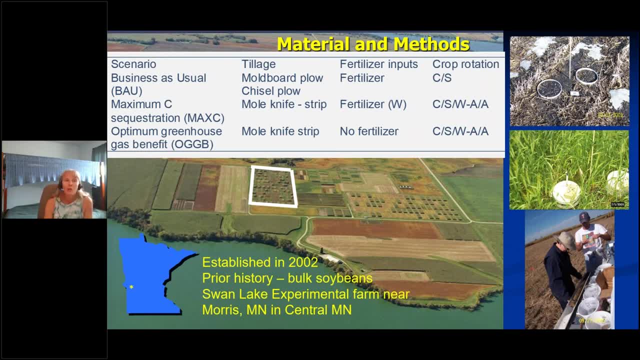 really trying to start getting a handle on what was going on in agriculture in terms of carbon sequestration- Was it being sequestered? How can we store more carbon? And we had delightful debates about what and how to measure. So in this particular study, we selected three scenarios. 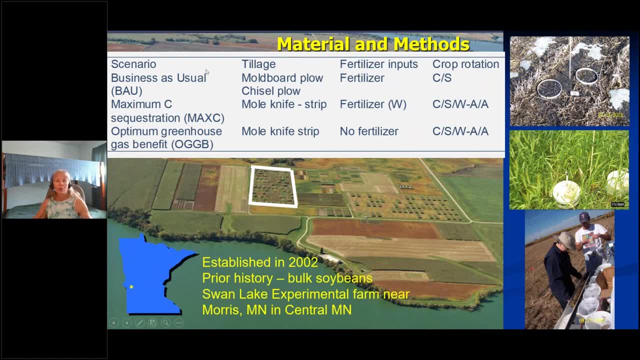 What was considered business as usual. So in Minnesota that was a corn-soybean rotation, Inorganic fertilizer- at that time I believe it was probably anhydrous ammonia- and then intensive tillage. We also had a maximum carbon sequestration treatment, which was a longer rotation. 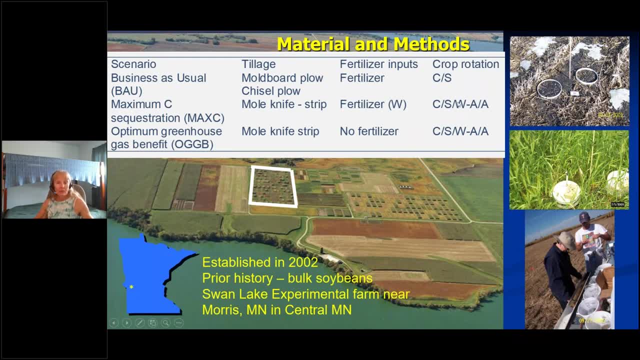 The only time it was fertilized was during the wheat phase. The corn relied on the nitrogen from the legumes in the system with reduced tillage. And finally, this idea of an optimum greenhouse gas benefit where there was no fertilizer applied, So the fertilizer or the nitrogen that was in the corn, it was not fertilized. So the fertilizer or the nitrogen that was in the corn, it was not fertilized. So the fertilizer or the nitrogen that was in the corn, it was not fertilized. The nitrogen for the non-legumes had to come from the previous legumes in the system. 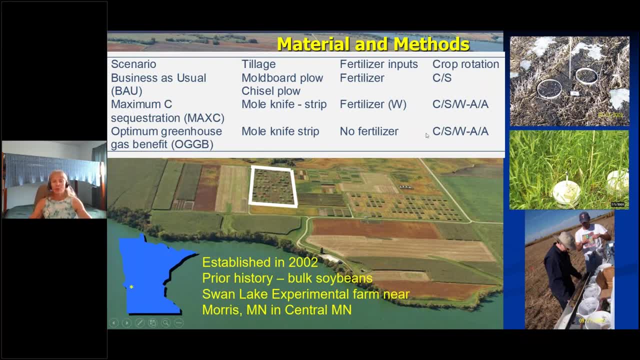 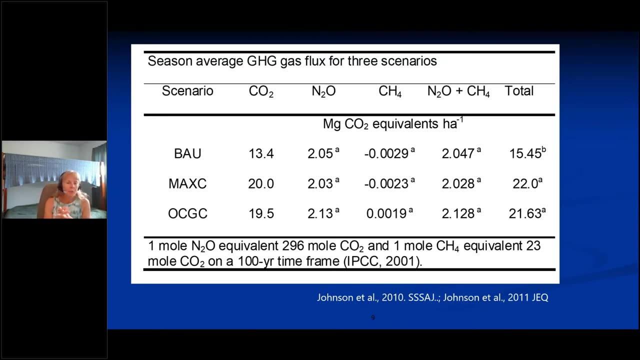 The idea being a fertilizer is a source of nitrous oxide that should reduce it, And the longer rotation should be increasing the carbon, And the longer rotation should be increasing the carbon. So if we sum this and take a look at it, this work has been published some time ago. 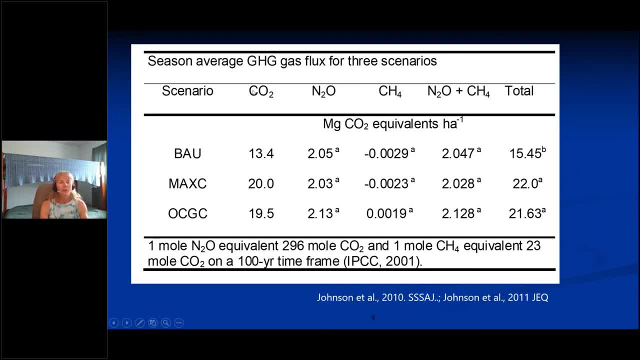 So, if we sum this and take a look at it, this work has been published some time ago. But one of the things you have to be careful of with carbon dioxide is that is that in these two systems, because we had wheat and alfalfa as soon as you put, 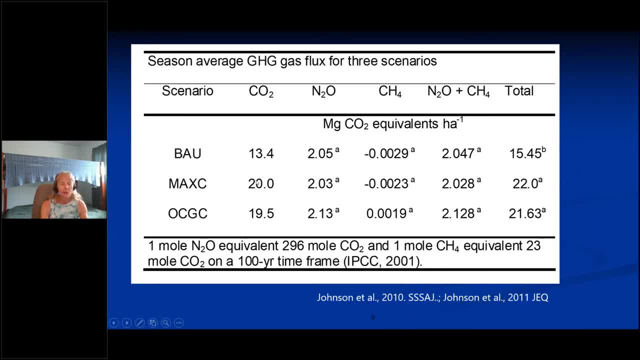 that chamber down, you're going to start getting erroneous co2 measurements. it's going to overestimate the site of the amount of co2 coming off compared to the business as usual, because you can put the chambers between those row crops rather than over it. as I had mentioned, the methane is very, very low. this is 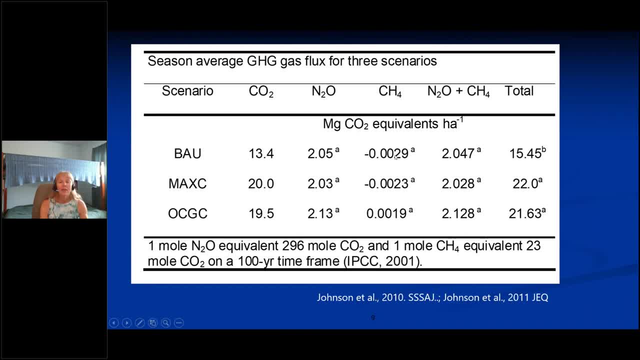 already been converted to mega equivalents and it's incredibly close to the detection limit of our equipment. so these are very small values and quite negligible when you look at, you know the multiple differences here. so, methane: we would have predicted that this, this would be the lowest treatment, but when? 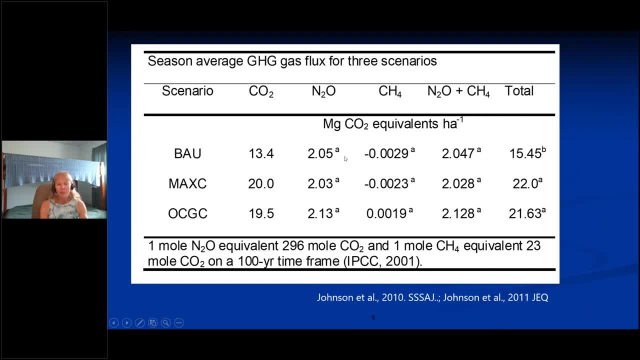 in reality, it didn't matter what the source of that nitrogen was coming from. we still had an in. you know the source of that nitrogen was coming from. we still had an in. you know the the about the same amount of nitrous oxide that came off on all three of. 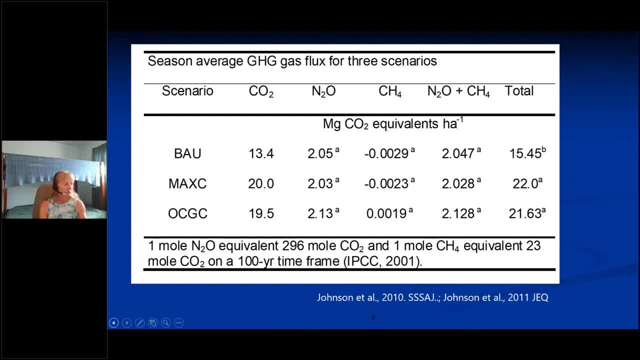 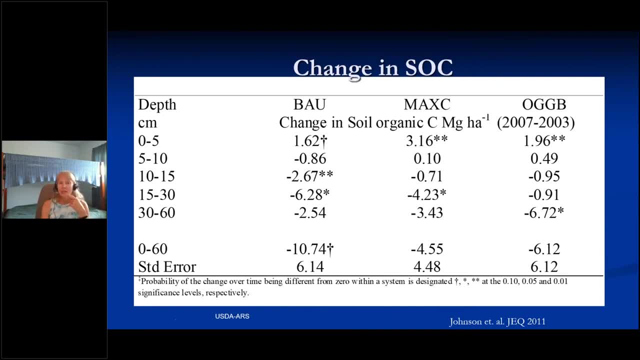 these systems. We also measured the change in carbons. We had a baseline carbon. We knew that had measured the bulk density so we could calculate on a- excuse me, calculate on a mass balance. So if there's so you needed, we needed to look at the change. 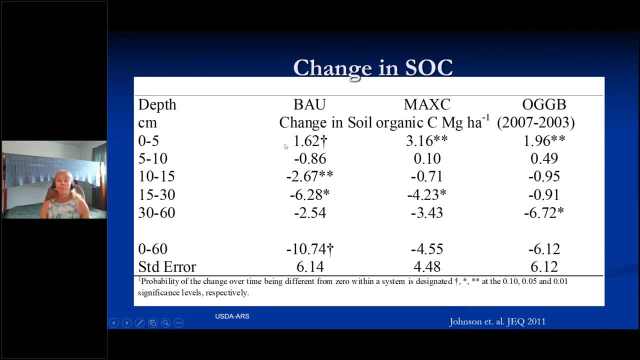 in carbon over time and not just among the treatments. So we were able to detect increases in carbon in all three systems, at least at the surface, but decreases at depth, so that overall the greatest loss was detected in the business as usual, but also some evidence that we may have been losing some carbon in the other. 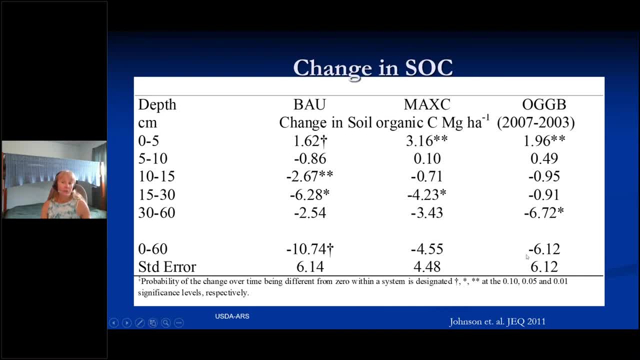 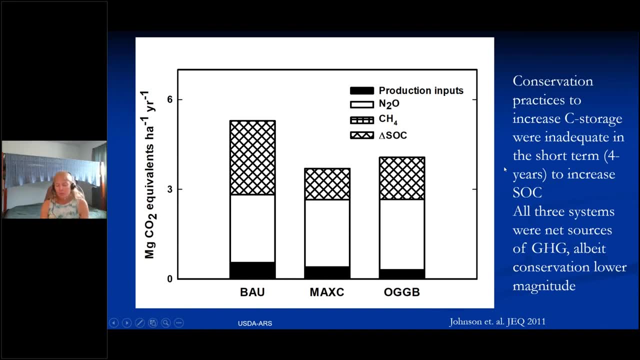 treatments as well, although statistically this is not different from zero, Similar to the graphs that Claire had shown. if we sum what's going on, so we have production inputs that would include things like the fuel that was put on and the fertilizer that were calculated. Those are the black bars here. 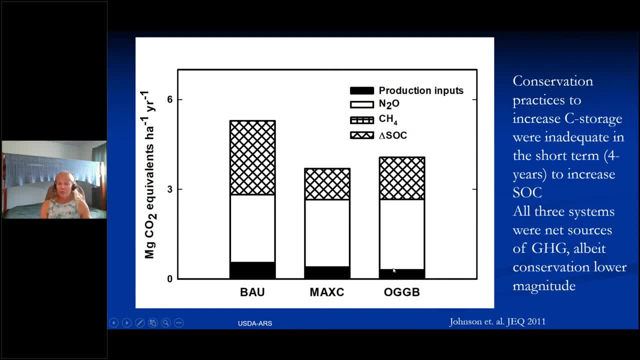 The methane is so small it gets lost in translation in the graph. Here's the nitrous oxide and then the loss in carbon. So in all three of these systems we were losing, we were going backwards. All of them were net sources of greenhouse gas. 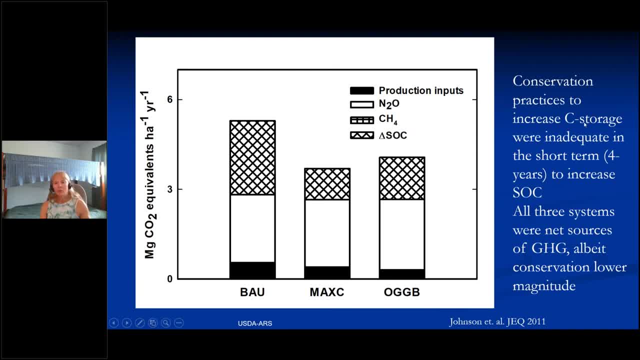 and we just were not seeing enough carbon storage to see a difference. Now, if we kept these going for another decade, considering how slow things change, would we? Maybe We could speculate that that may happen eventually, But nonetheless, you know the we didn't see zero, but at least it was. 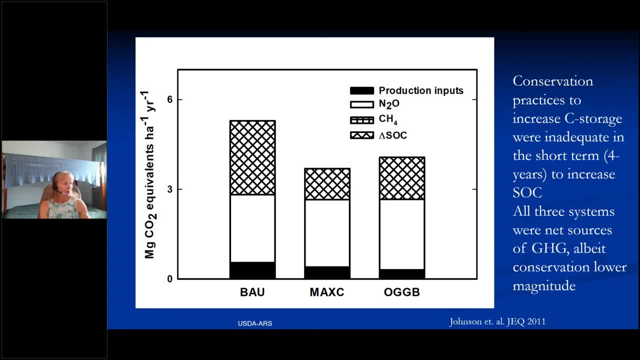 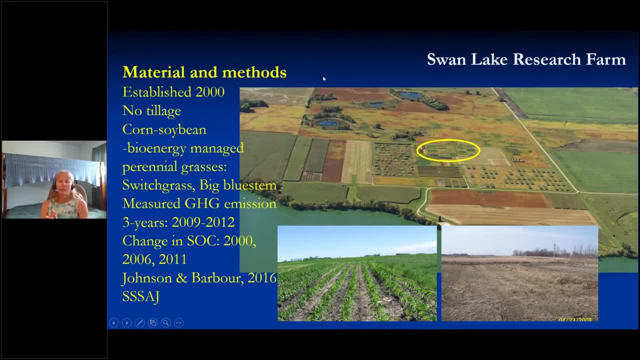 less. So I guess that's that's what we're trying to do. So I guess that's what we're trying to do. So I guess that's a positive sort of Not going to get us to net zero, though In another study that we did that on a similar type of system, the plot so was. 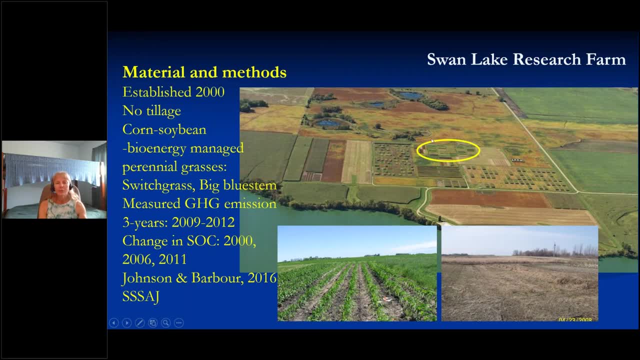 talking about for over here now we shifted. these plots were established in 2000,. they had been in no tilling since then. It's a slightly wetter area on the field Again. we have corn and soybean cereal, which is quite popular and you score proper beans but they depend on gym and water. my 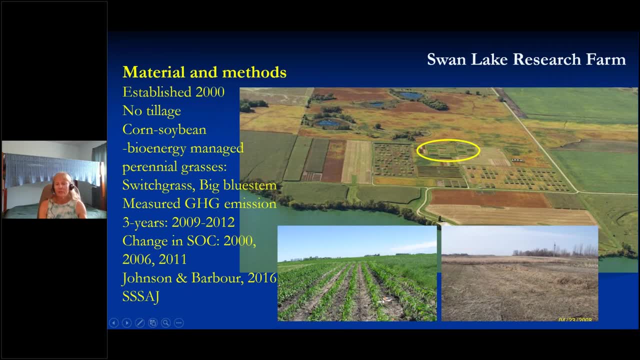 Again. we have corn and soybean cereal, which is quite popular, and you score proper beans, but they depend on gym and water- my soybean as our baseline system. Here's the chambers and alongside we have perennial grasses. These were being managed for biofuels, so these were intensely managed grasses. They were not. 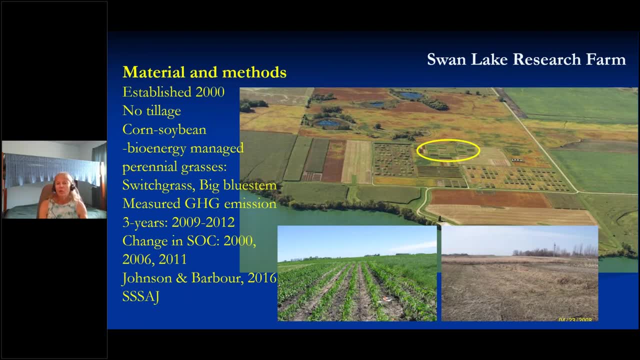 trying to mimic a native system. They were looking at this from the context of bioenergy, which ideally bioenergy would shift to biogenic use of carbon rather than fossil carbon. but you have to be careful not to cause problems with your soil organic material as well. 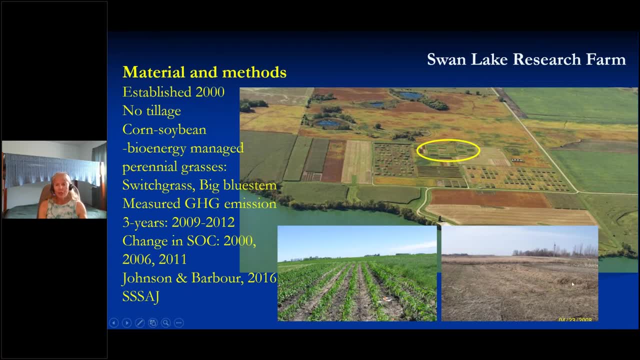 The big bluestem or the switchgrass would be harvested either in the fall or in the spring. Then we monitored the change in carbon. We had baseline numbers. We had them in 2006,, which was done shortly before we started measuring the greenhouse gases- and then inclusive. 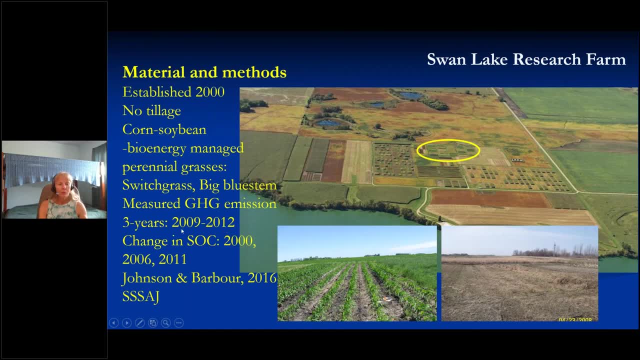 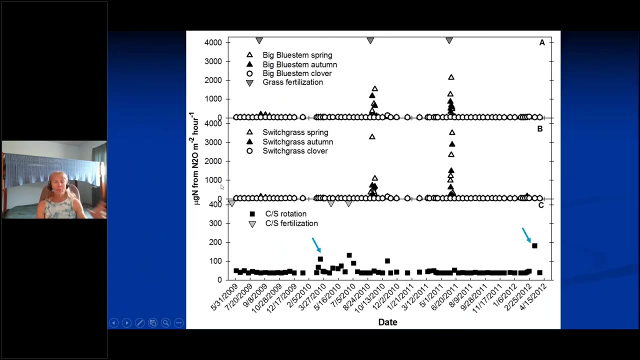 of a fall sample in 2011 and we measured greenhouse gas for three years. This work has been published in SSSAJ Soil Science Society of America Journal in 2016.. So this gives you a nice example of the kind of messy stuff you get when you go. 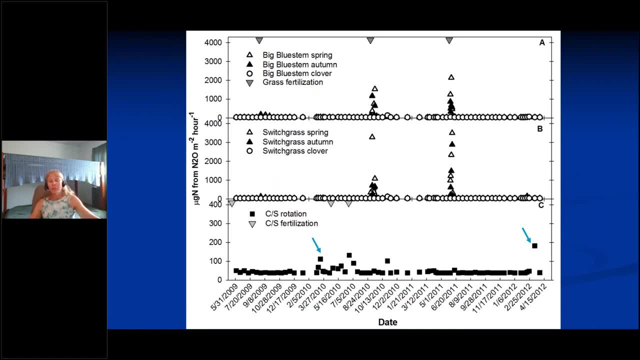 out in the field and you try to measure nitrous oxide with with closed vented chambers. You spend a lot of time out in the field and you come back, you bring them in and you're at or near the detection limit, Interrupted by spikes. 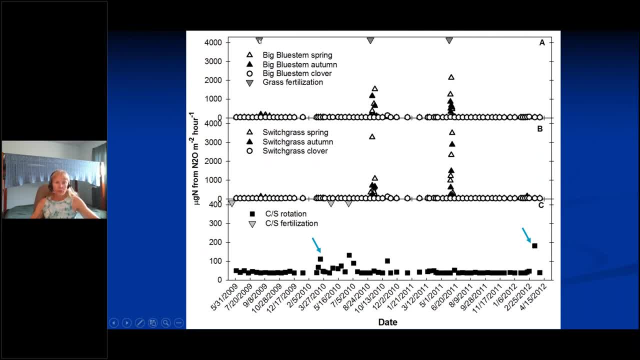 that are caused either by fertilizer events, which are signified by the gray arrows across the top, And the other event pointed out here with the blue arrows are spring thaws. Now, this is, as I mentioned. we're in a northern climate. It gets very cold. 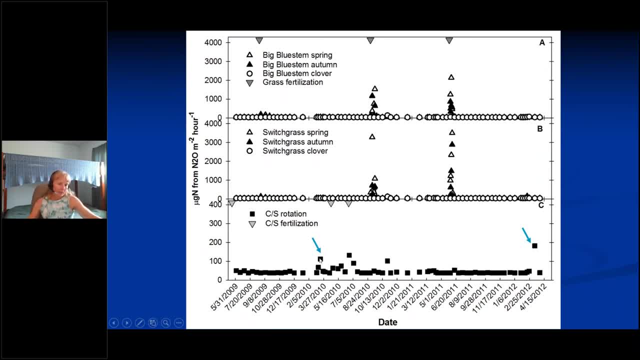 We tend to have snowfall and in the spring, sometimes before you have true flux in terms of total thawing, you get the soil surface thawing, you have disruption of the cell contents of anything may have been there. you have nitrogen available, you have a soluble carbon and you get. 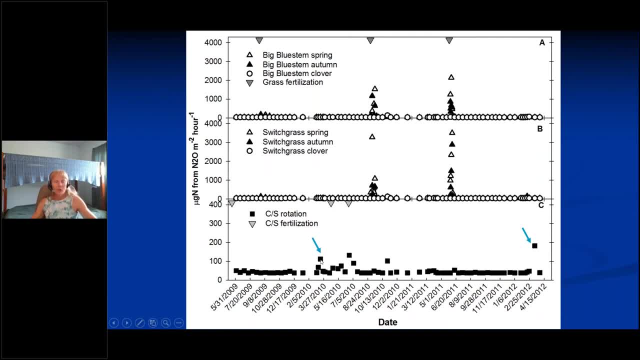 these spikes in in nitrous oxide coming off, Interesting though we didn't see that in our perennial grasses We see the impact of the fertilizer. Like I said, these were intensely managed, so they were fertilized and depending on the climatic conditions, the weather conditions of the time, 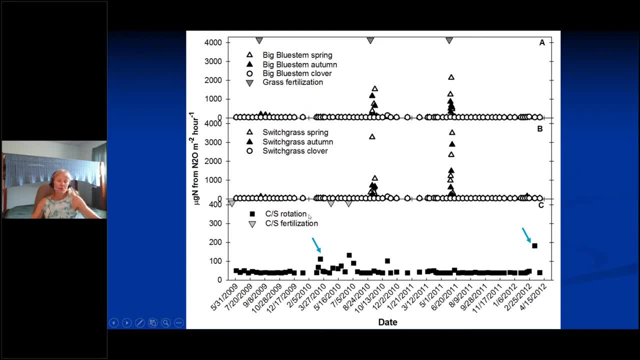 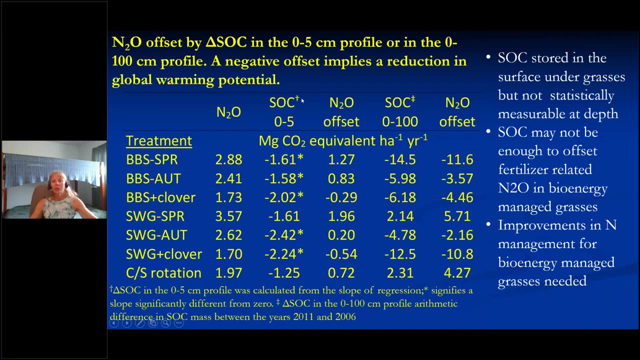 the spike from the fertilizer could be quite variable. If it was dry at fertilization, you don't see denitrification and pretty limited amount of nitrous oxide coming off those systems. We also measured the change in carbon, So the carbon that was stored under the grasses. 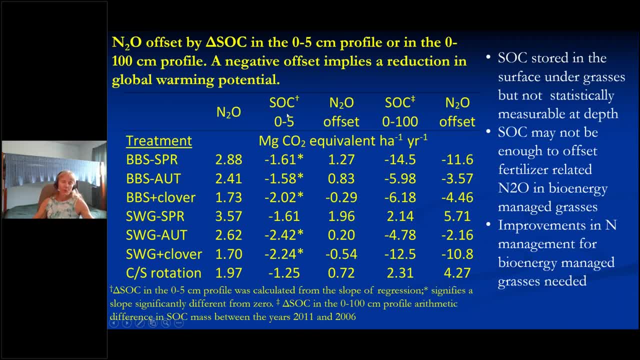 again, these were managed so that residue was being harvested every year, so we're not seeing a huge buildup in the amount of soil organic carbon that was there. We had some storage, particularly significant, at the surface under the grasses, but not under the corn. 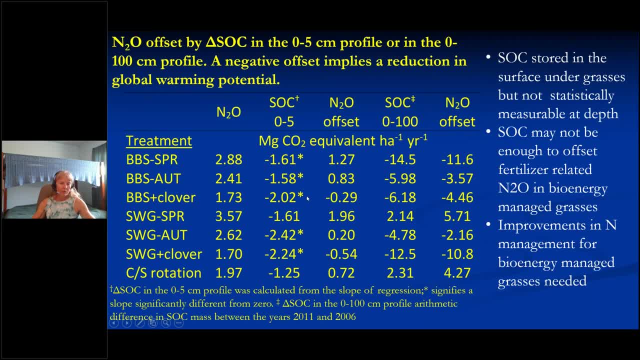 And soybeans. the star means that it was a significant difference based on the regression line for those. so from time one to time three and regressing that data. So if we look at those again, a negative offset implies a reduction in the global warming potential. 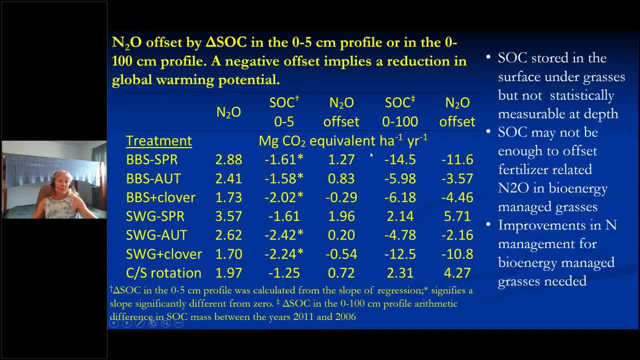 If this is real, then perhaps we are getting an offset. but the difference in the change in carbon was not significantly different, So we're not seeing a significant shift in carbon from zero, although it is encouraging to see its least going in the right direction. Perennial grasses did not guarantee that this was going to happen. 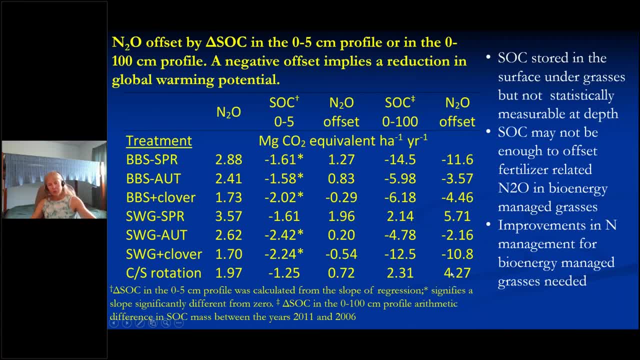 Depending on when we harvested, there seemed to be an influence of the management of those grasses, and the corn and soybean certainly was the greatest emitter. even though this isn't a significant difference, It does not bode well and that is, I guess, as predicted. 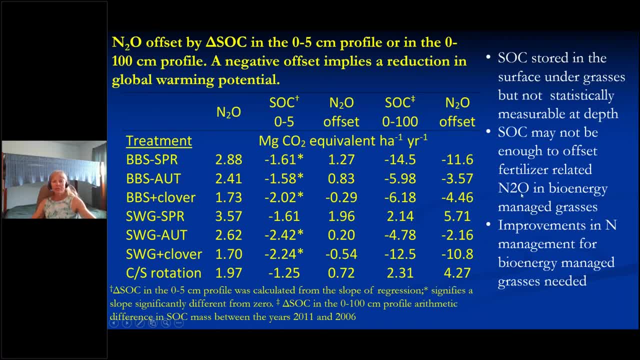 Even though it's not a significant difference, it does not bode well and that is, I guess, as predicted. Even though it's under no-till, we're still having a positive influence In terms of the nitrogen management on these switchgrass treatments. there is an opportunity. 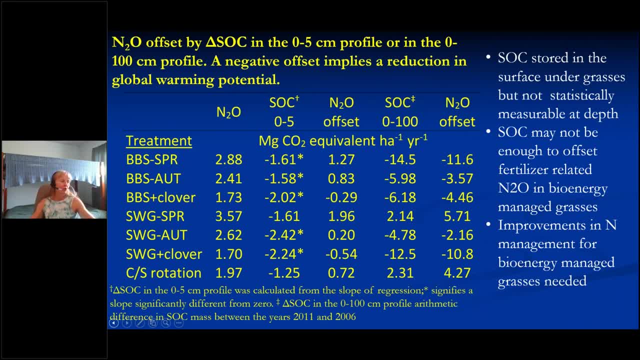 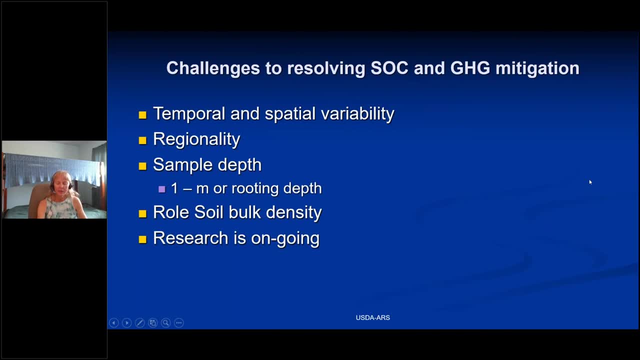 here that I think we can do some improved management with the nitrogen fertilizer on those crops to improve those numbers. So if you're trying to really get a handle at what's going on in SOC and greenhouse gas, you have to deal with the fact of temporal and spatial 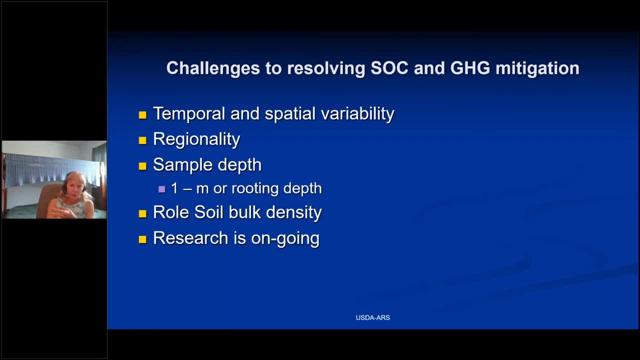 variability, and that's true for the nitrous oxide, it's true for the soil, organic carbon, And accept the fact that you're going to have trade-offs. if you're trying to really delve into good temporal data, You may do that at the risk or at the expense of spatial 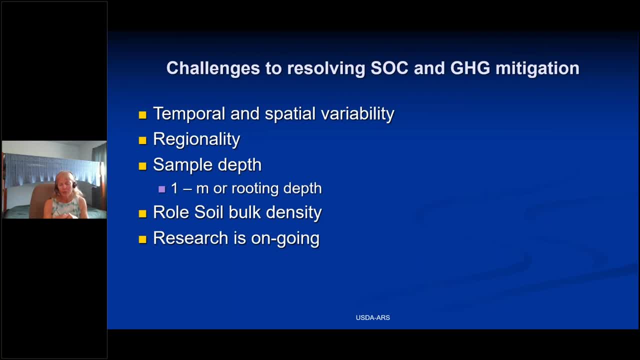 values, The new nitrous oxide sensors that are coming online, that we're hoping to install yet this year- better temporal values on what's going on with nitrous oxide. but it will be on one farmers field and one cropping system, so alone it's a case study, but it 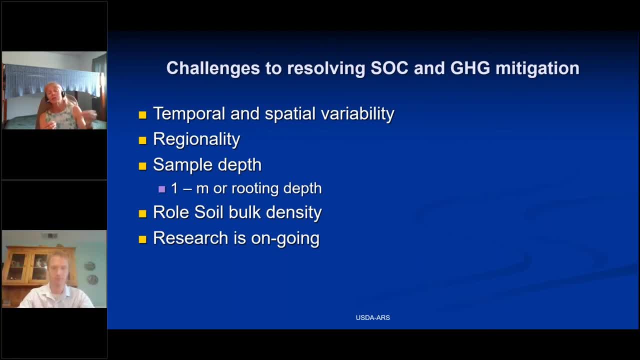 will have to be coupled then to other studies across the region using this type of technology, and what works well here may not work as well someplace else. bulk density is highly variable, the depth is important and there's a lot of ongoing research through ARS, university partners and in the international. 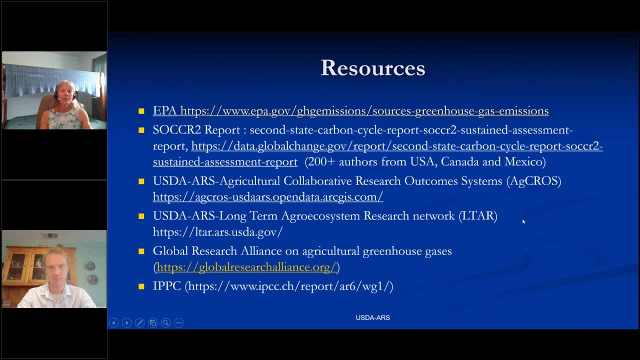 community. I just want to leave you with just of a list of some of the resources. when I look through some of the questions that Claire Phillips had shared, that people had submitted, I was impressed by the depth and the depth of the research that they shared and I think it's a good way to. 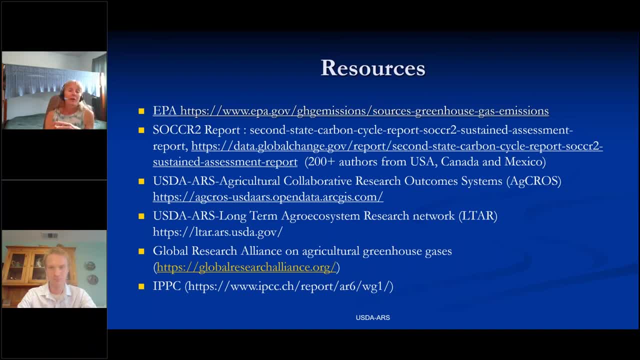 understand the extent. there are some incredible resources that are publicly available, including the work that's done by EPA. I have ARS scientists that help with the modeling components of that for trying to get a handle on what's going on on our greenhouse gas inventory on an annual basis- the soccer to report. 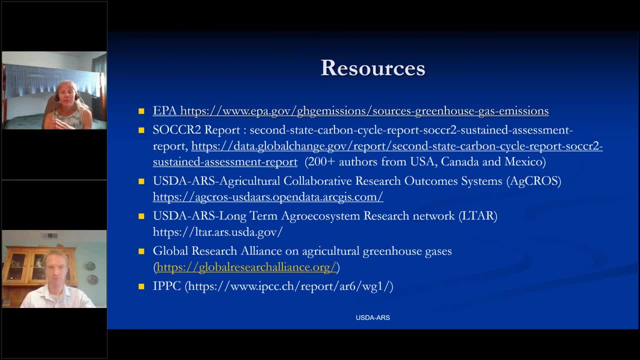 included over 200 authors from the United States, Canada and Mexico went through very intensive review and internal and external review. I'd like to bring to your attention the USDA ARS agricultural collaborative research and outcome system, AG cross, if you're looking to just get a feel for where the studies are in the United States, it's a 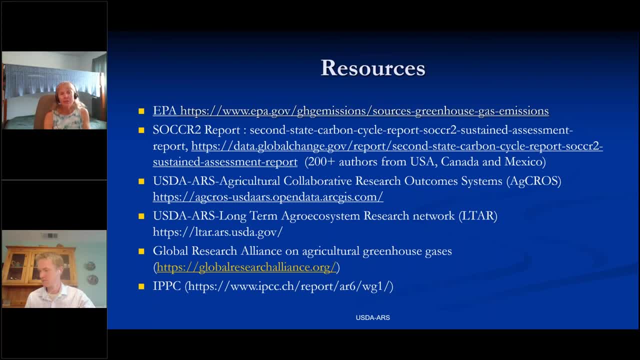 great opportunity: a lot of data that's housed there. the relatively new- although it's been around now for for about five years- is a lot of research that's been done in the United States, and the United States has a lot of research that's been done in the United States, and the United States has a lot of research that's been. 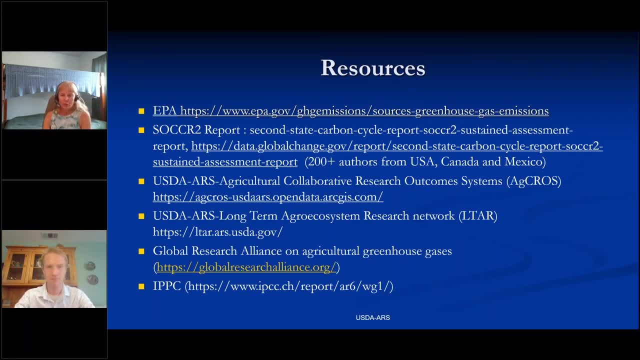 the USDA agriculture long-term agro ecosystems research network and they're really trying to get a handle on what is sustainable- how do we balance the inputs- and it's looking at grow crops, it's looking at grazing system- so it's very broad- and figuring out ways how to bring this data together during 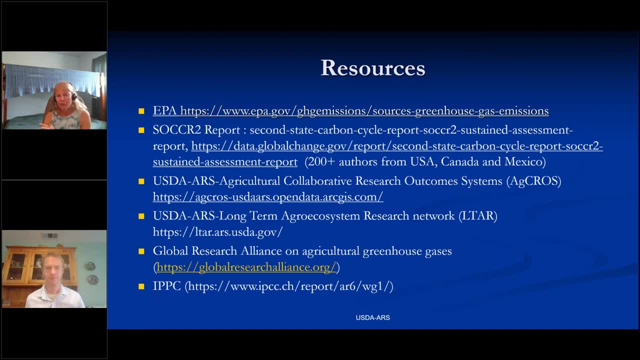 my introduction they had mentioned the global research Alliance on agricultural carbon, our agricultural greenhouse gases. Last I looked, I believe they're up to over 90 participating countries. It also has a great set of resources on how-to, some training videos that are available, so I'd encourage checking it. 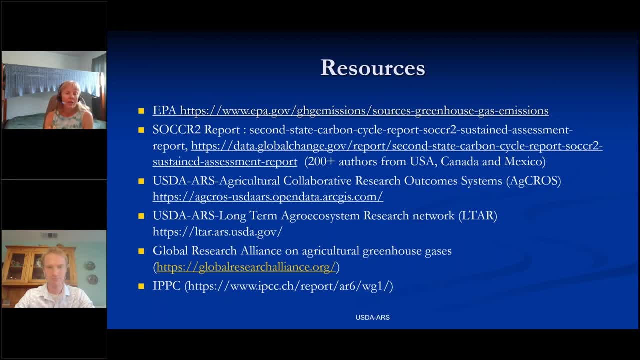 out if there's a group that the working group on livestock. there's a working group on cropping systems, Patty Rice, with really phenomenal research and opportunities for the cropping systems and I believe it may extend into the livestock. There's Magnet, which houses the 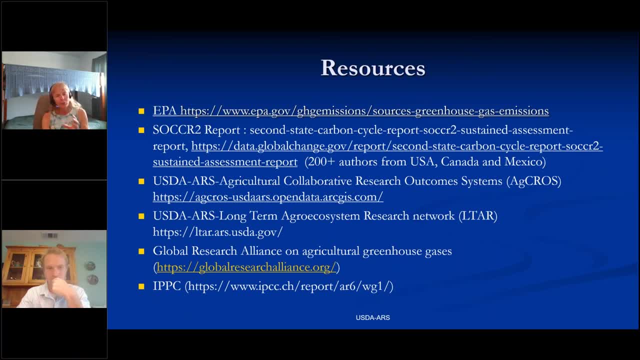 metadata for many of the studies that are available to help people get an idea of who's out there doing the work. and, of course then the IPCC, who's been around now for a good long time. They just came out with the new annual report. 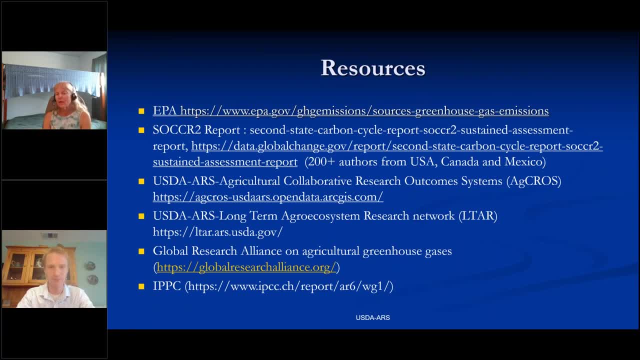 New report, number six, and I know it's gotten some media play and I have not had a chance to really go in and dig into it. but again, an incredible resource for those that are interested in climate change and trying to understand how do we find these answers Earlier this spring. 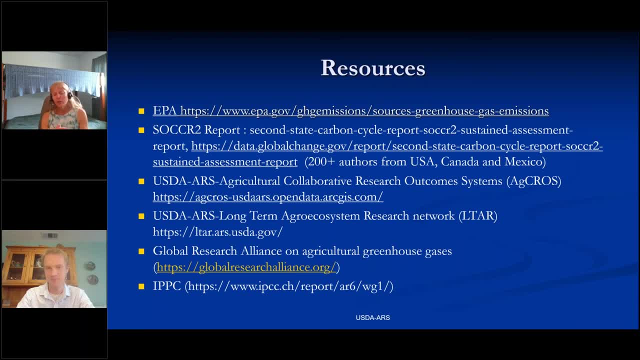 or this year, I was part of a network orchestrated to discuss how do we achieve net zero, and there's a lot of work that's being done on that. There's a lot of work that's being done on that. There's a lot of work that's being done on that. 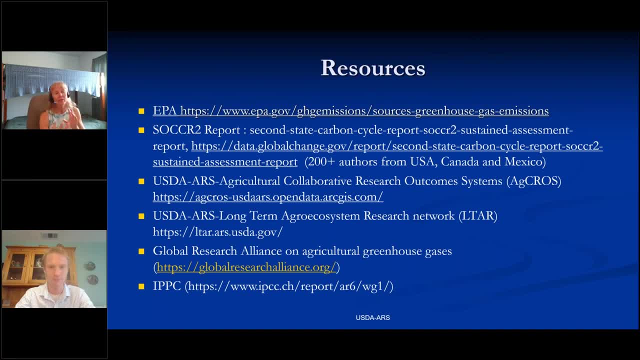 And so you know what research questions can ARS and our partners help answer. So it is a very timely subject and I applaud the organizers for putting this together and very excited to see the number of people that are attending. And with that I'll turn it back over to you, Eric, to cover any questions you may have. 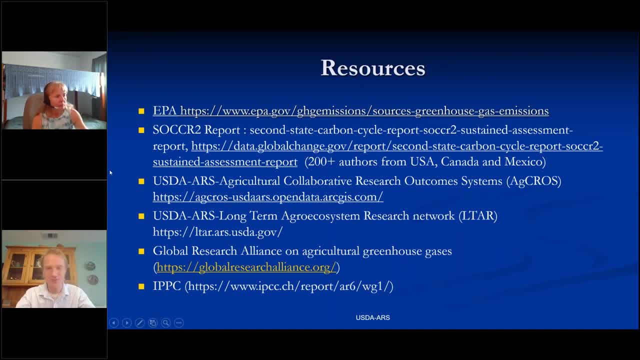 Thanks, Jane, That was terrific. It was great to delve into some of those case studies that Claire was mentioning earlier and could see the complexity of the different outcomes. in these systems often things don't seem to respond the way we expect or that we hope perhaps. 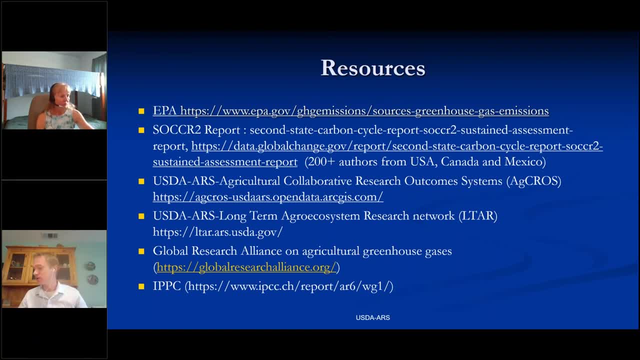 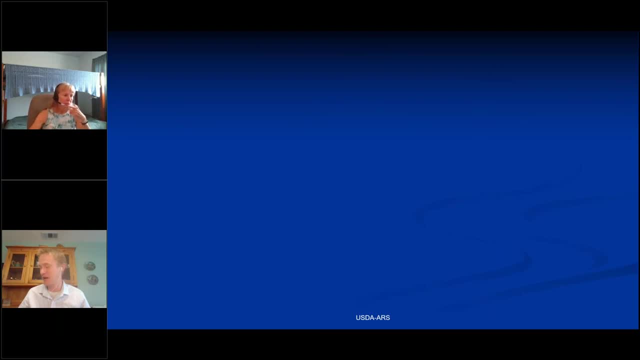 But let's see in terms of questions, one question that came up: this is almost a philosophical question more than it is a scientific one, perhaps, but depends on how you look at it. Global warming potentials are referenced to different timeframes. 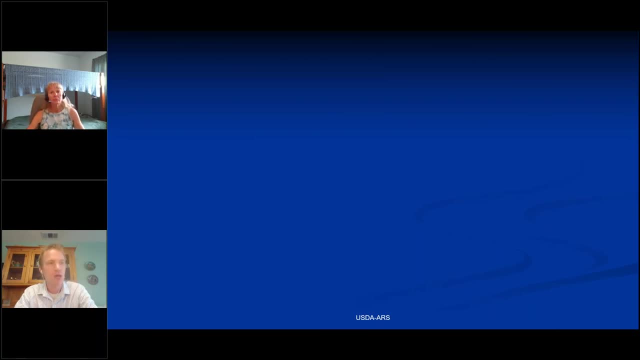 This is something you mentioned earlier on in your talk. So what does it mean to pick a particular timeframe for calculating global warming potentials, And do you have thoughts about whether a 30-year versus a 100-year timeframe is more appropriate? And what do we mean when we communicate that way? 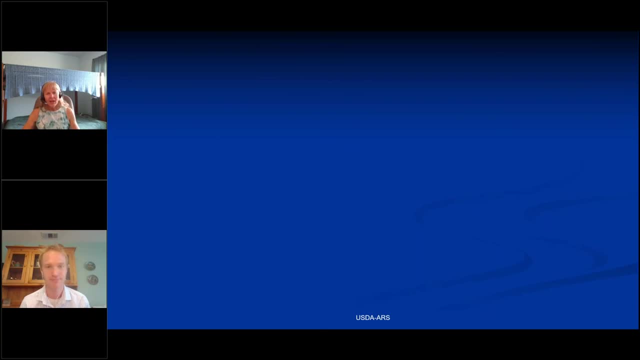 by choosing a temporal reference point. I'm not 100% sure. I do know that the most common one I see is 100 years- And I mean 30 years makes sense because we can understand what may happen and we can think about. 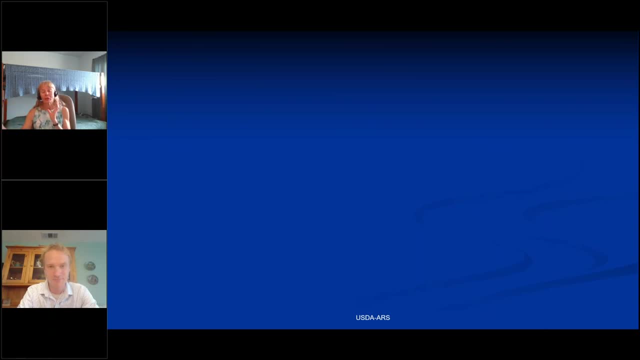 we maybe can get our hands around 30 years. 100 years sounds like a long time. Most of us are not going to make it for 100 years, But I think if you want to have extended change, then the 100 years makes sense. 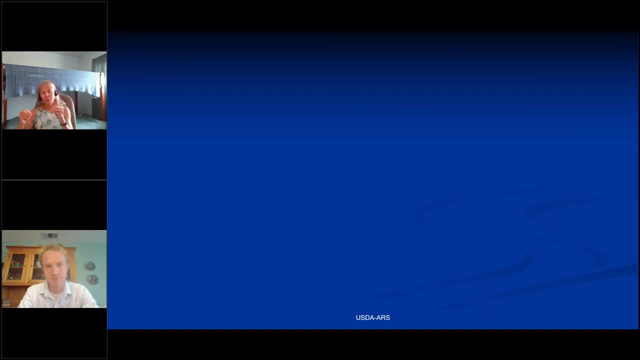 And if you dig into the IPC and they do have a chapter that explains the rationale behind this, how those numbers come in. And some gases don't last long. They have a very short lifetime. CO2 has a very long lifetime in the atmosphere. which is one of the reasons it's used as the benchmark. Nitrous oxide has a fairly long compared to methane, which is shorter, but it also is constantly being produced, So I think it again. it comes back to what is the question you're trying to answer. 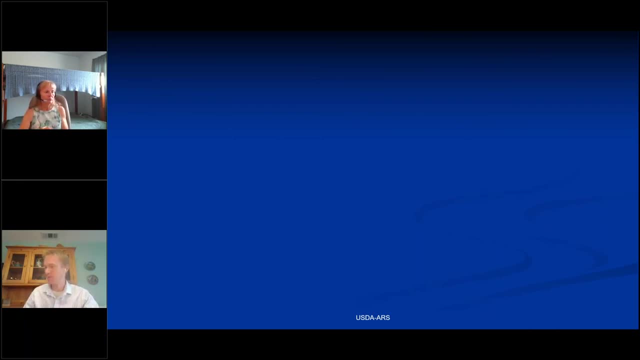 What is the question you're trying to answer? Great Thanks, So another question that I was thinking about, and that relates to some of the other questions we received, is about climate. At various points you talked about the thaw events and the N2O related to those thaw events. 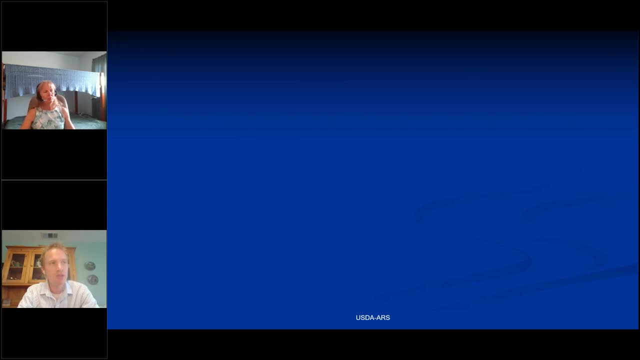 And I'm wondering: are there particular climate domains that are more susceptible to N2O emissions, say snow-dominated climates, for instance? Do you imagine that the concerns might be different in warmer climates farther to the south? Oh, absolutely. 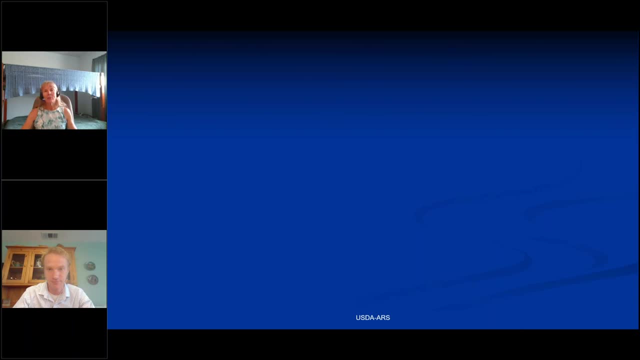 The spring thaw event really is a phenomenon of soils that freeze and thaw. I have colleagues that you know in Indiana, for example, and even though they were out there looking for those events, they didn't happen. There's work that's come out of Germany, where they've seen it. and some other northern climates. So if you have these thawing or freezing cycles, where the soil is frozen at depth and then they thaws back out, you're more apt to see it If you have very mild winters, there is no truth. 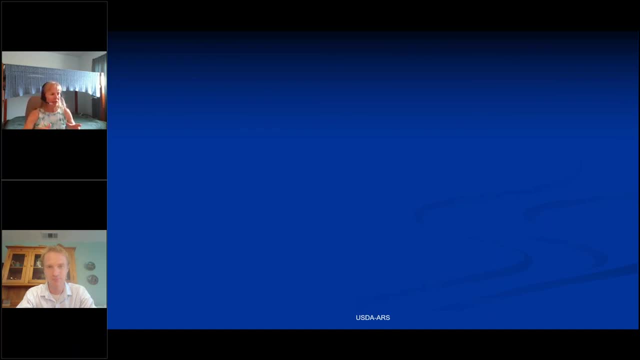 Yeah, There is no true thawing event. that happens And kind of colloquially, what I envision is happening is that soil's frozen And if I was going to predict today to see nitrous oxide coming off of a field in a northern climate like Minnesota, 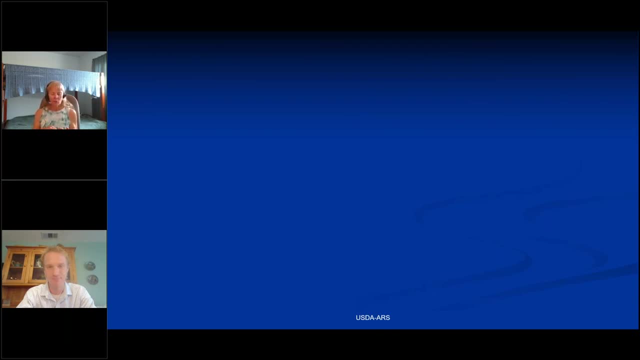 it would probably be mid to late February, on one of those days where the sun is out and intense and you get this slimy slurry about. I don't know. I don't know. It's about half an inch or a centimeter in depth. that's thawed. 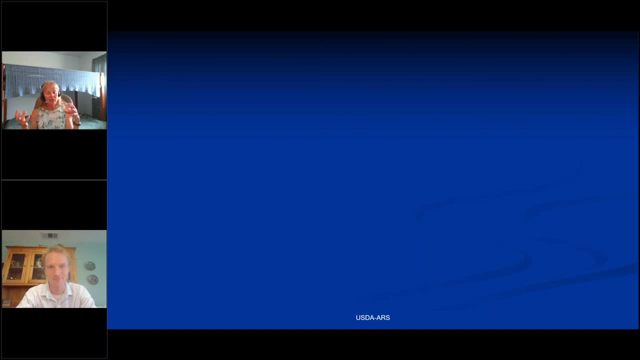 And so the water can't go anywhere. It's denitrifying, It's cold. The only place for those and those microbes are. you know, they're awake, It's warm enough for them to go, And so they're chewing up whatever is available. 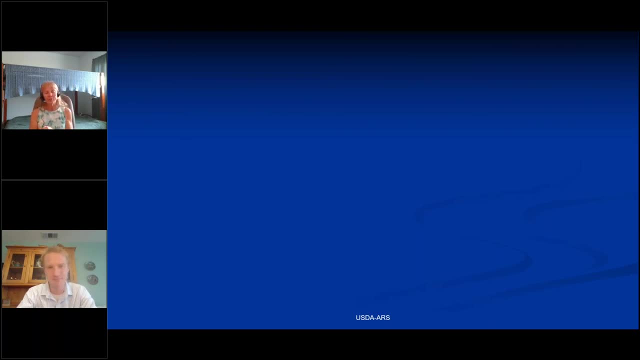 and it's denitrifying. So you have all this nitrous oxide come off and it freezes again at night and everything stops And the next day it may happen again. So it's very ephemeral But it can be 30 to 50% of the nitrous oxide. we've measured out in those fields for the course of the year. 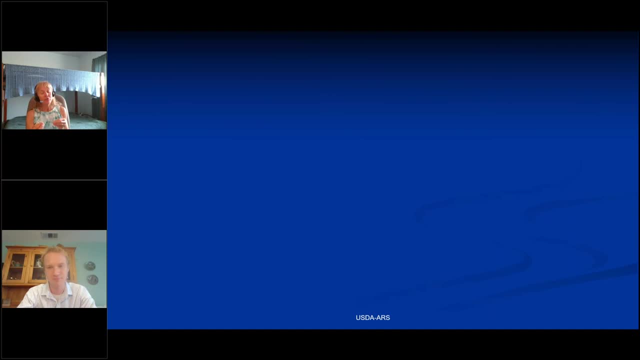 So it should not be neglected. It's difficult to model because it's so ephemeral. It's difficult to measure. So I'm excited when we get this new sensors coming in out at the field to really get a better handle on what might be coming. 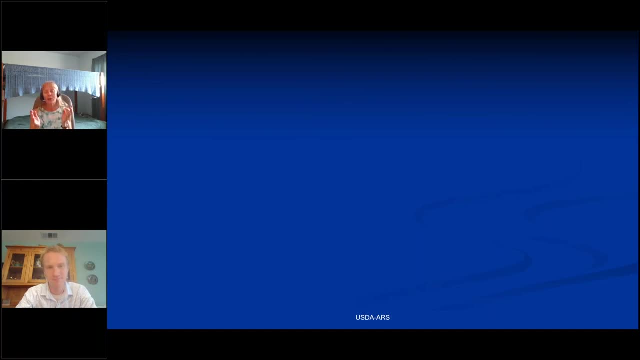 even though it is a one spot, but we will be able to look more closely at those temporal variabilities. Good question, I like that one. Yeah, it's very interesting. Just a brief follow-up question is, given that it's an ephemeral event, perhaps that's encouraging because it gives us something to target right. 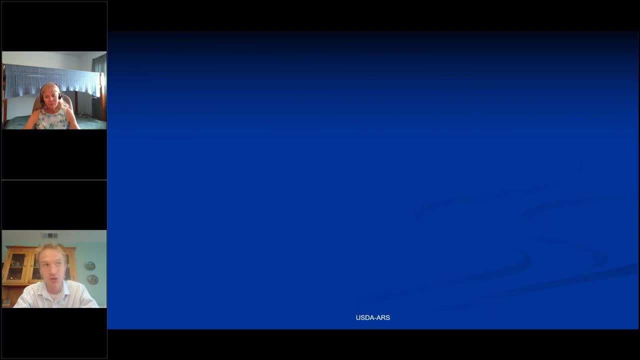 But are there management approaches that can target that Brief window? Or is it really out of our control? because the soil is going to thaw and if there's nitrogen available, what will happen will happen. Is there a way to prepare for that event? 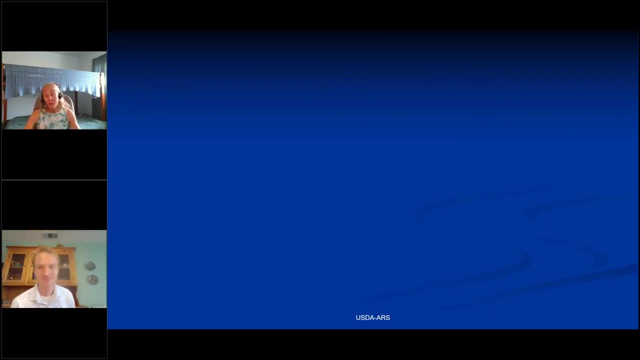 It really is. I don't know that there's a way to prepare for it per se. If you have a source of nitrogen in that soil and it freezes, you're going to have some nitrous oxide coming off. It does come back to the importance of making sure that you 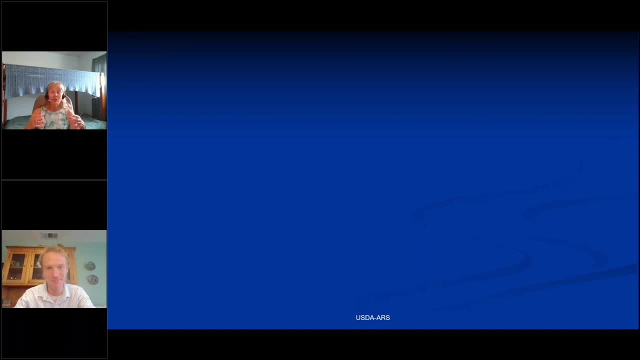 And some of it might fall into this indirect I mean. if the nitrogen didn't get used up, it's sitting there in the materials on the soil And then you get this freeze-thaw event. You have a source of nitrogen, You have a source of carbon. 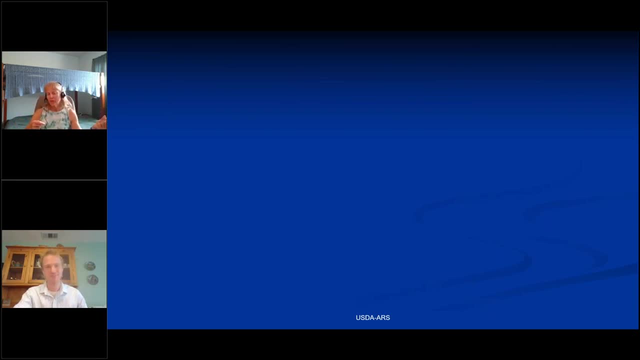 What is intriguing is that when we looked at it in those perennial systems with the grasses, we did not see the same flux that happened. They're covered, They're protected, They're free. It would be an interesting, It would be an interesting study to very carefully go in and measure those temperature gradients that may be happening under those systems compared to a more bare soil. 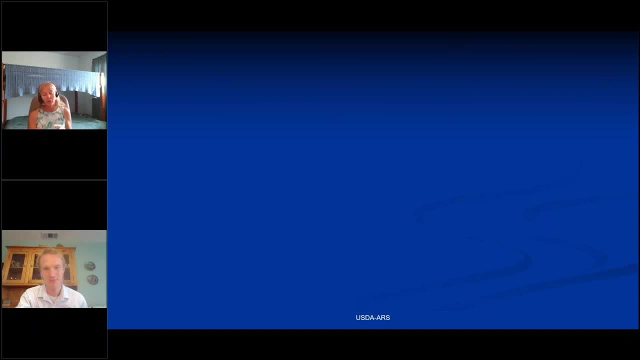 We know that the microclimate, for example, is going to be quite different under those perennial systems than what they are, And that would be a grassy system rather than a legume compared to a row crop. So I think there's lots of research questions still available.